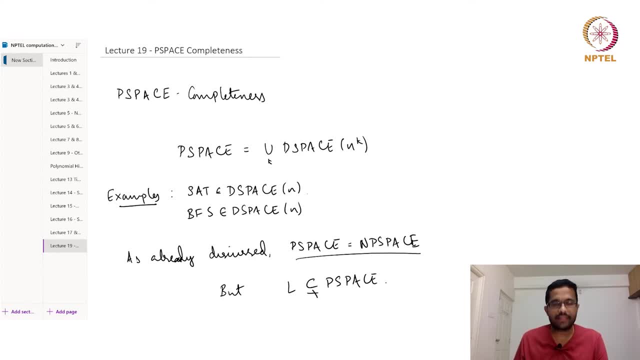 complexity class, which is based on the space usage. So this is p space. So what is p space? It is just a space analog of p. p is the. p was the set of all the languages that could be solved in polynomial time, Whereas p space is a set of all languages that could 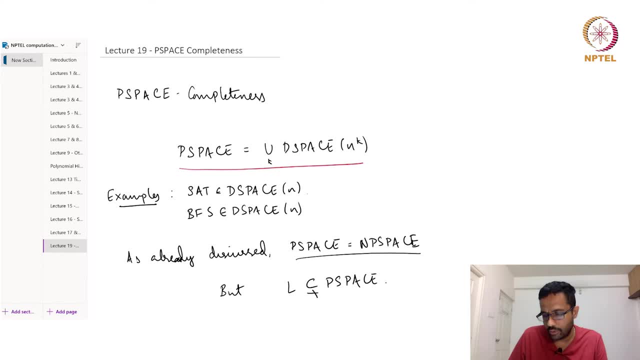 be solved in, that could be decided in polynomial space. So it is a union of d space, n power, k, So for all integers, k. So maybe I can say k equal to 1, to infinity, So anything that can be solved in any polynomial space. 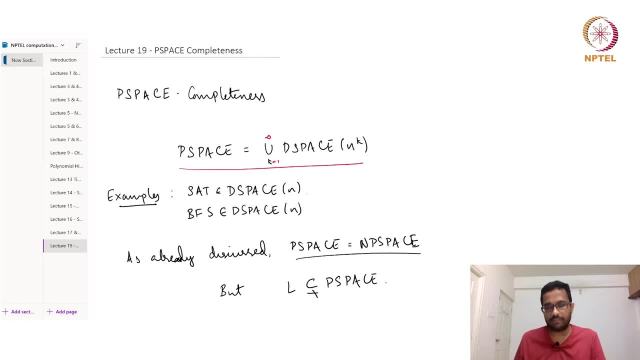 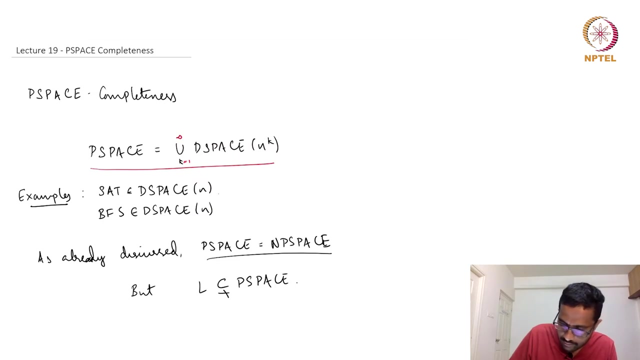 So p space is in p space. So, as we have seen, just to remind you, d space of fn is always contained in d sorry d time of fn, is always contained in d space of fn. Hence p is contained in p space. What I am saying is that you we have already seen in one of the previous 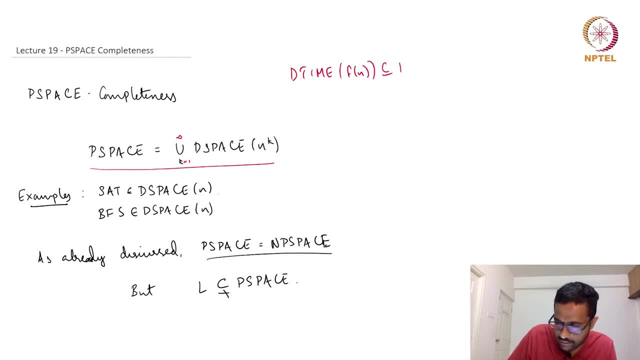 lectures. So d time of fn is contained in d space of the same function. Maybe I will just move it around here. So hence p is contained in p space. So if something can be done in fn amount of time, It can certainly be done in fn amount of space, just because in one time step it can write. 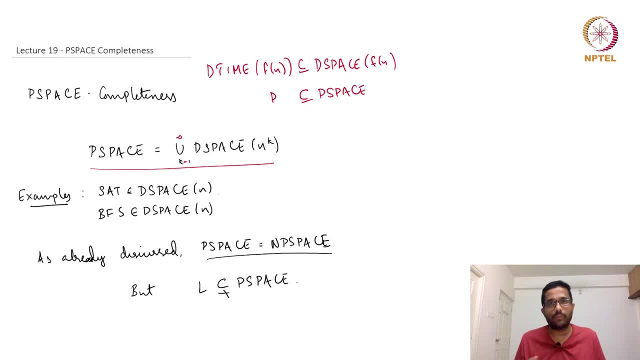 at most one tape location. So the space usage will never be more than the time taken. Anyway, this p space is. p is contained in p space. This is an easy inference. Some languages that are in p space are, let us say, SAT, for instance. So, given so, why? 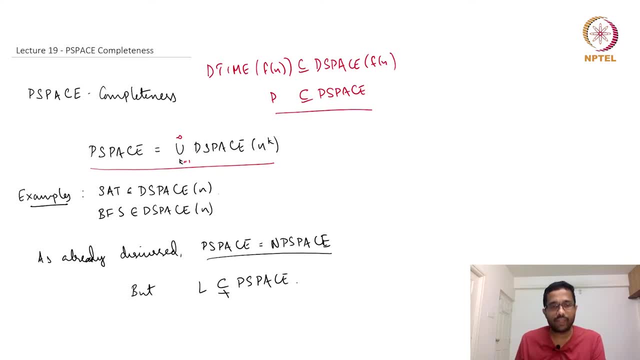 you SAT in P space. I did not write as well as how a simple GET in, but this is how I in fact sat is in linear space. Why is that? Because, given a particular assignment you could have, so there are n variables, let us say, and, which means there are 2 power n possible. 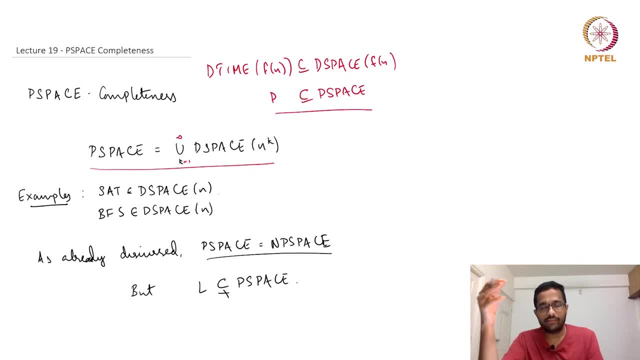 assignments. We could have a counter of length n where we cycle through each of these assignments and we try out these assignments one by one for the Boolean formula. And verifying a Boolean formula whether a certain assignment sets it to true or false is not that difficult, So that does not take any significant amount of extra space. 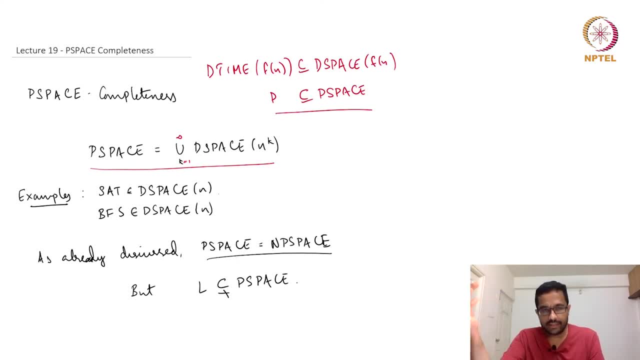 So all the main idea is just this. So the space required is linear space. Similarly, maybe if you consider breadth first search, given a graph and you want to do the breadth first search, it is also linear space. So because the graph itself in adjacency list representation. 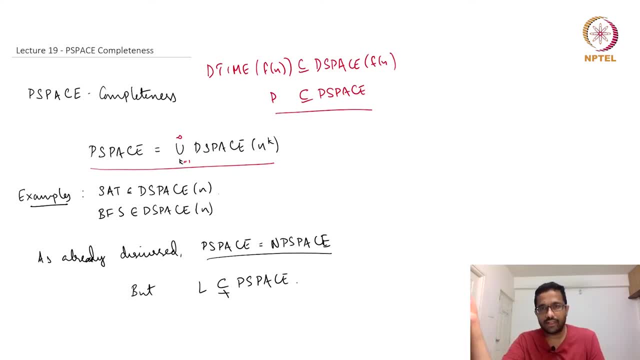 requires order n plus order m, where sorry vertices plus edges and whatever is required for the representation of the graph is it is the time required. the space required for the BFS is linear in that, So BFS is also d space n, So this is not that difficult to see. So 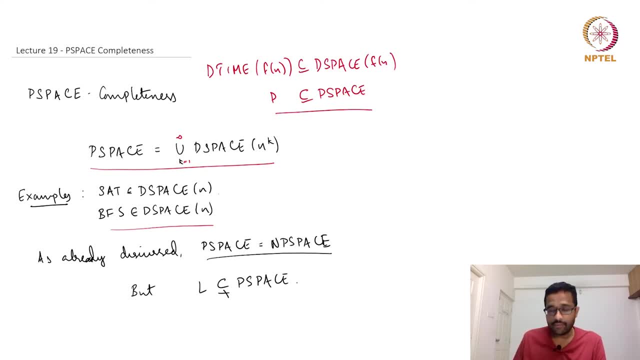 I am not going to elaborate further on them- And we have already seen that p space is equal to np space, meaning if I had defined a non-deterministic analog of p space, it is the same as p space itself. So this is something we do not have in time complexity. 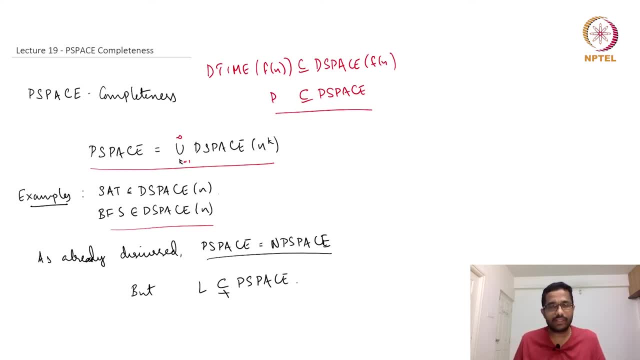 p is different from, or we do not know whether p is equal to np. that is a big problem, big open problem. But whereas in space, complexity, p space and np space are the same, Again, this is yet another example of things happening in space differently than how they used to happen in time. 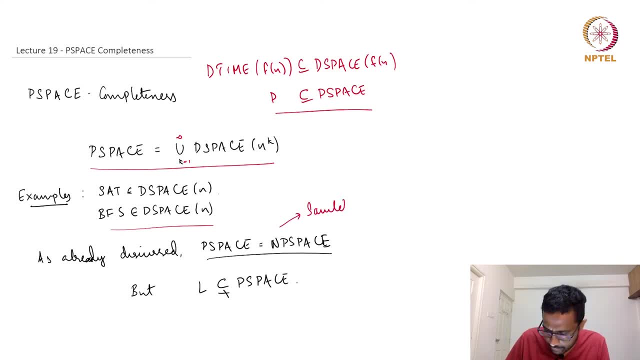 So why is this? This was because of Savitch's theorem. So any polynomial, let us say np space, so clearly p space is subclass of np space. but then take any non-deterministic polynomial space machine. you just square the polynomial that is the space usage of the corresponding 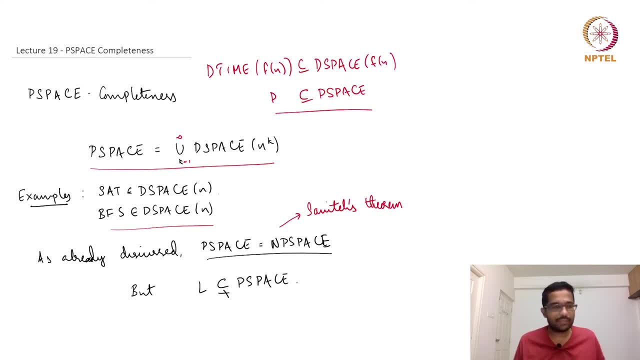 deterministic polynomial space machine. So it will just be square of a polynomial. square of a polynomial is still a polynomial. So something takes n power k- non-deterministic space. it can be done in n power 2k- deterministic space. So if n power k is a polynomial, 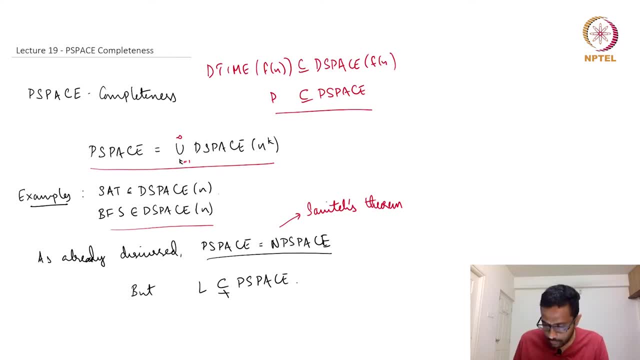 n power 2k is also a polynomial. However, the class log space is distinct from p space. Why is that? This is because of something that we are yet to see called space hierarchy theorem. So it is kind of similar to time hierarchy theorem. So what it says is that so time hierarchy is a. 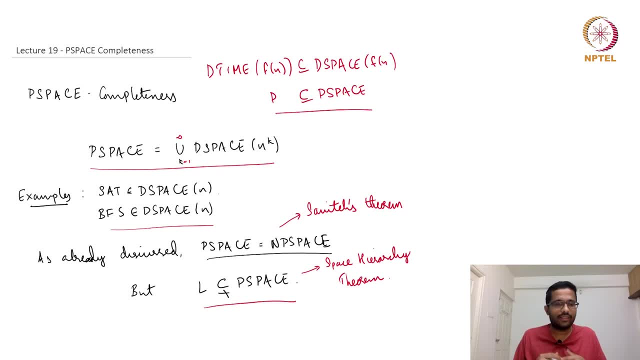 polynomial. so time hierarchy theorem kind of said that up to some logarithmic factors, if you have two functions, f1 and f2, d time f1 is strictly contained in d time f2, where f1 is smaller than f2, then d time f1 is strictly smaller contained in d time f2,. 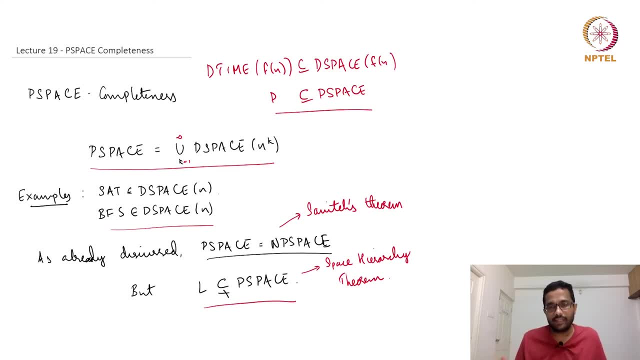 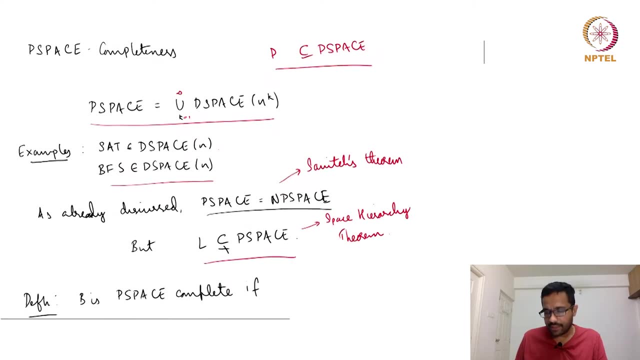 meaning there is some language that it can be decided in f2 time which cannot be decided in f1 time, as long as f2 is sufficiently bigger than f1. Something similar we can say for space also. we will soon see this. the proof not in this lecture, but in an upcoming lecture. 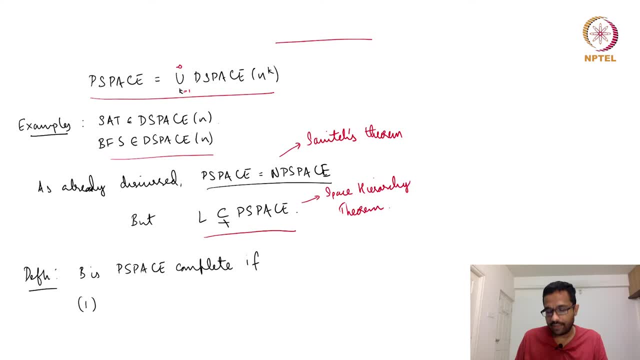 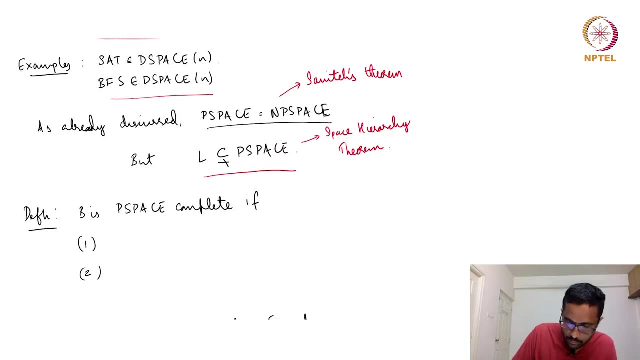 So here we have log space in the left hand side and we have p space in the right hand side. So that is a distinction. Now let us define. so again, this is just some aspects about space, complex p space. So now let us define p space. 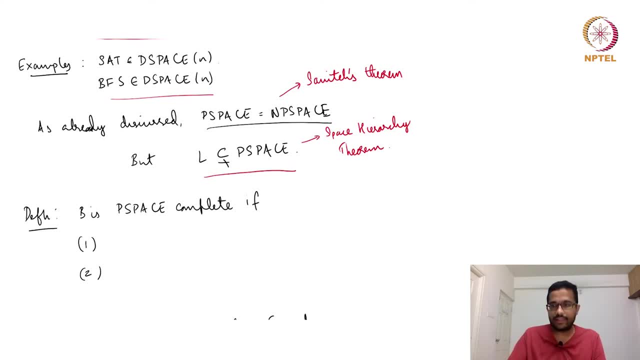 completeness. Again, this is similar to. we have already seen two notions of completeness in this course: NP completeness as well as NL completeness. so this is yet another notion of completeness. Just like what we have seen before, it uses reductions. So let me formally define it. 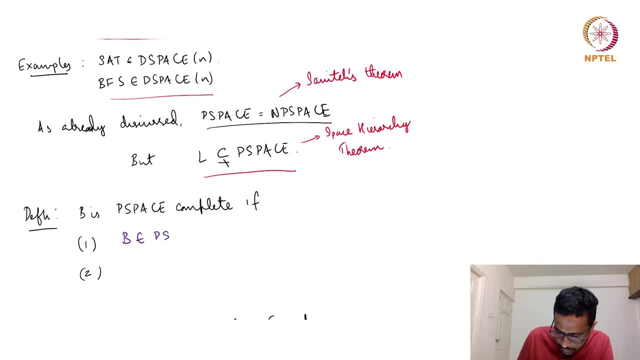 The first part is simple: b is in p space, b is p space complete if b is in p space. just like we said, b is NP complete if b is in NP. And two: every p space language, every language in p space, for all a in p space. 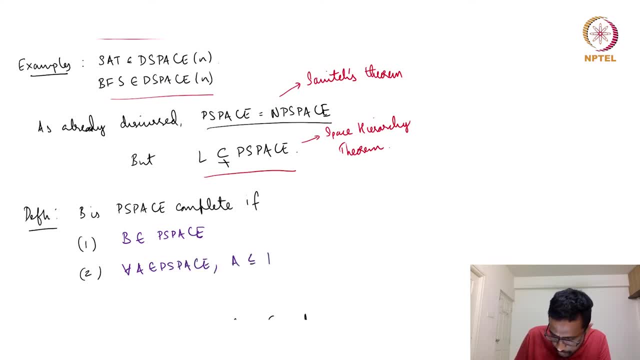 a is reducible to b, But what is the reduction used? So, in the case of p, in the case of NP completeness, we had polynomial time reduction. In the case of NL completeness, we had log space reduction. So what is the reduction used here? So one thing. 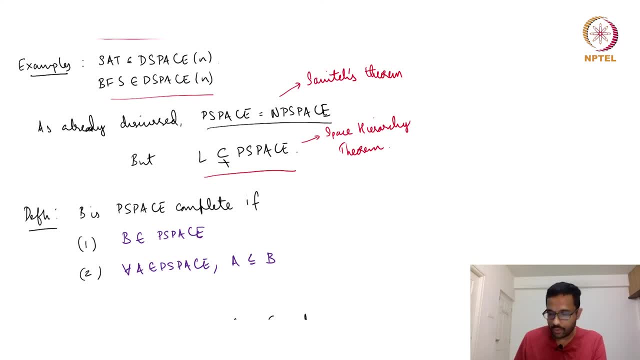 to note is that the reduction used, the reduction used should not be as powerful as the class itself. So we cannot say p space reduction here, because then it would mean that if any a is in p space, if you use p space reduction also, then you can, you might, as. 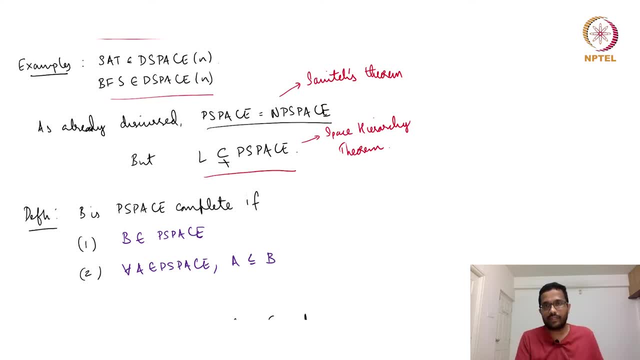 well, decide the a, you do not need a reduction to transform it into another thing. So, in fact, in the case of p space completeness, the reduction used is just what we have already seen: it is polynomial time reduction. So as of now, 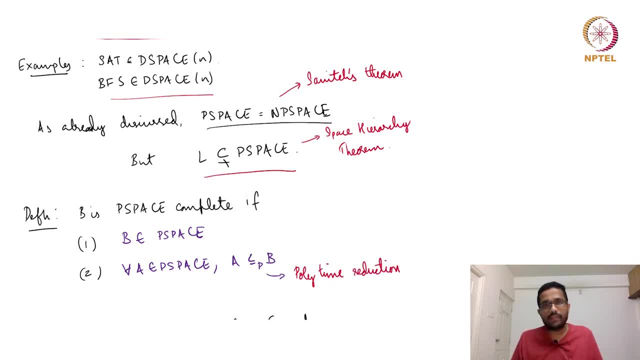 Now we think polynomial time is not it is. we do not know if it is as powerful as polynomial space reduction. right, It could be lesser powerful, but it could be the same too. That is why it is. we find polynomial time reduction to be appropriate to use for this requirement. 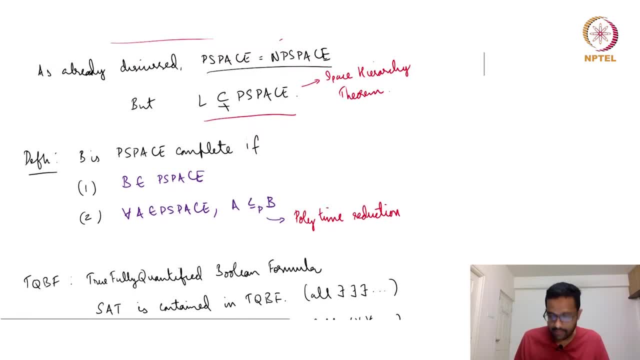 So it is something that is that seems to be less powerful than p space, right? So again, we have already seen polynomial time reduction, right? So now let us. this is p space completeness, Now, let us see. now, let us see a p space complete language Again. 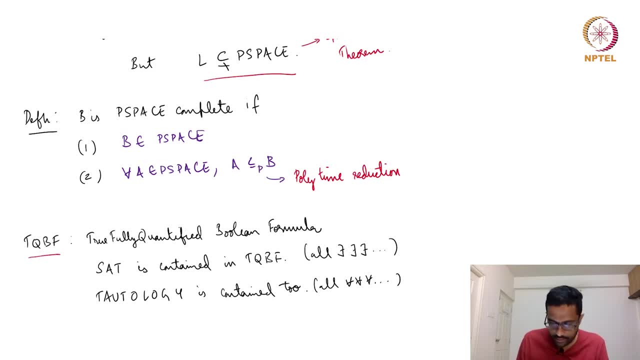 whatever I am saying, it is there in CYPSR. The language is called- maybe I will just say true- fully quantified Boolean formula, or it is otherwise called TQBF. So what does it mean? It is a Boolean formula. However, in the case of satisfiability, right or in, 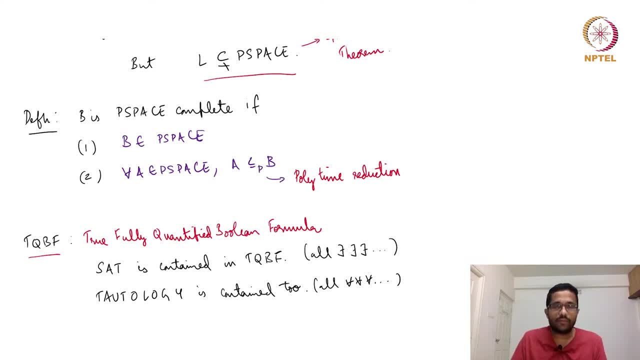 the case of tautology, We also had a Boolean formula, but there the requirement was different. right, In the case of SAT, if I gave you a Boolean formula, you had to decide whether there is some assignment that SAT is that sets the formula to true. In the case of tautology, the question was: 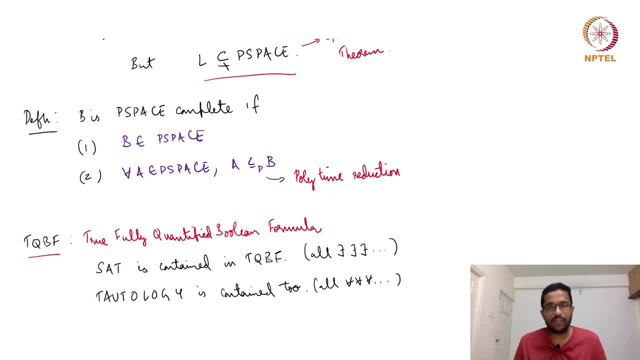 is it the case that all the assignments set this Boolean formula to true right? So one is asking: is there some assignment that makes it true? Second is asking: do any assignment does it make it true? Both of these can be viewed as fully quantified Boolean formula. 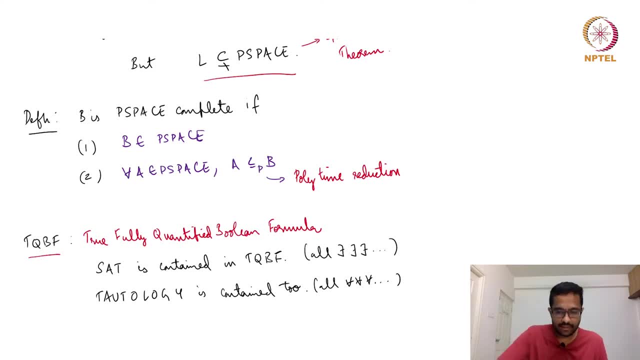 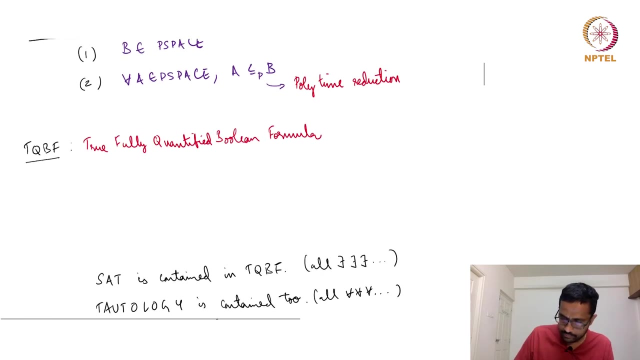 right. So what is fully quantified mean? Suppose there is a- maybe I will just write this right- Suppose there is a fully quantified Boolean formula. right, Suppose there is n variables. there is a formula psi with n variables. right Now, a fully quantified. 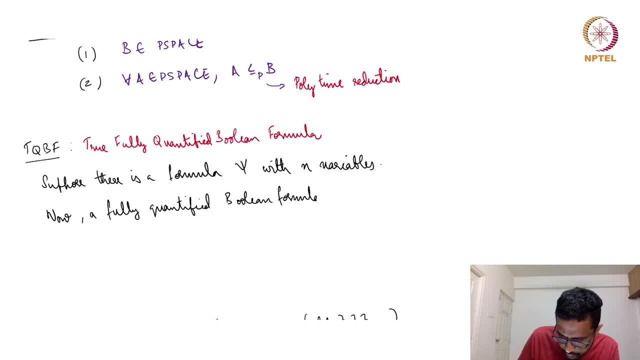 Boolean formula, right? So what is fully quantified Boolean formula Or fully quantified psi, is of the form q1, x1, q2, x2 and so on: qn, xn. So let us say the n variables are x1, x2 up to xn, and then psi, where each one of these q1, q2 are. 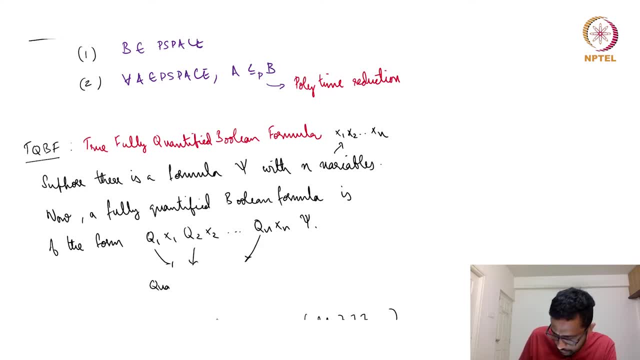 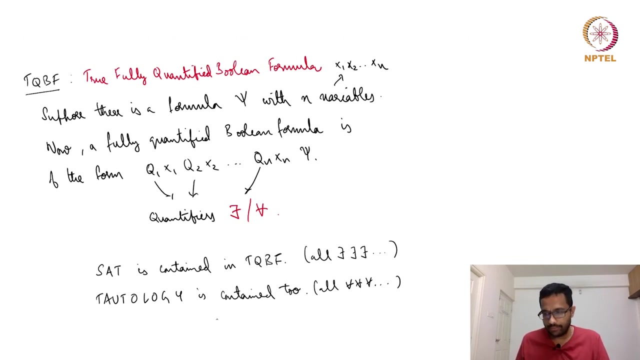 there, they are all quantifiers. Quantifiers mean they could be existential quantifier or universal- sorry, or universal quantifier there exists or for all. So basically now, what is SAT? in this form, SAT is a fully quantified Boolean formula where we are asking: does there exist an assignment? 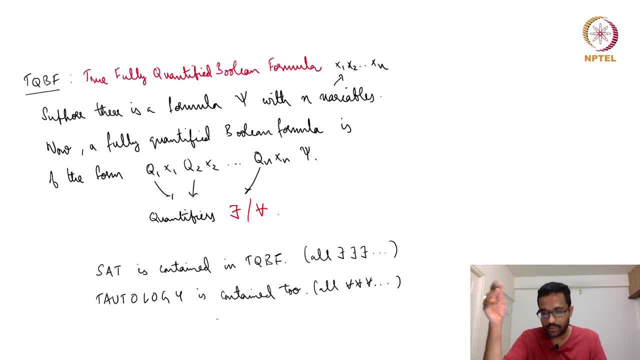 such that all of these are set to. the formula is set to true, So we could think of it as where all this q1, q2, etcetera, all of them are existential quantifiers. right, If all these q1, q2 are, we are asking: there exists x1 such that there exists x2 such that there. 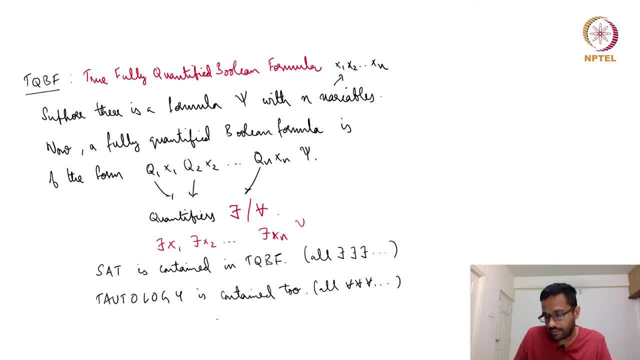 exists xn right, such that the formula is true. that is satisfiability, Whereas tautology is something where all the assignments right, So x1,, x2, etcetera, all the assignments for all the variables set to, sets the formula. 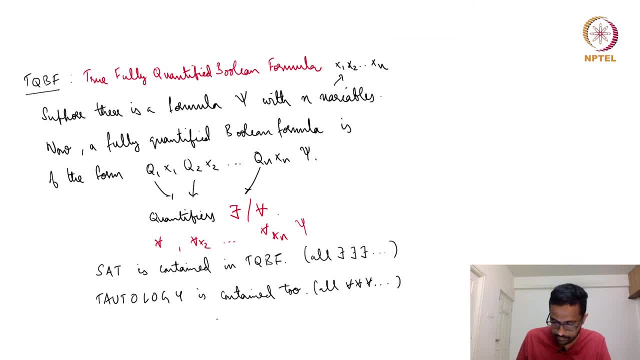 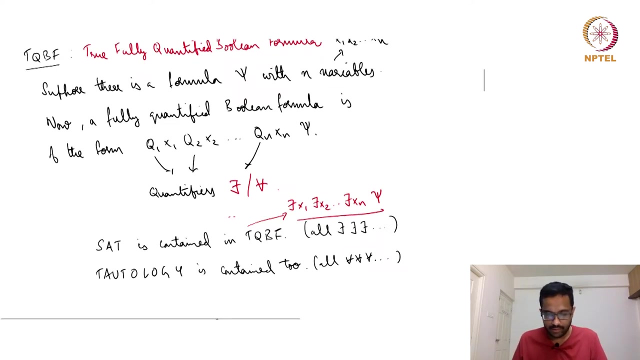 to true. So it is a for all situation. Maybe I will just so. SAT is something like this: there exists x1, there exists x2, there exists xn psi. right, this is SAT, Okay Okay. So both tautology as well as satisfiability are TQBF And if you think about it, we saw 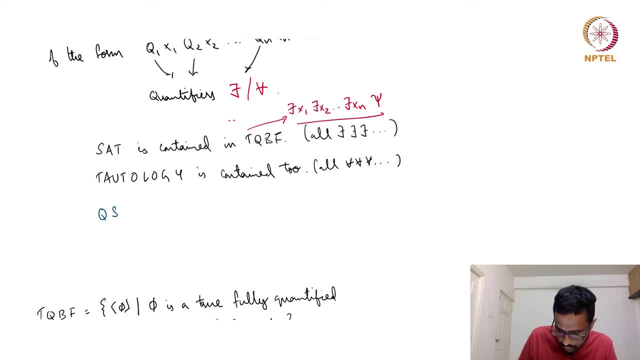 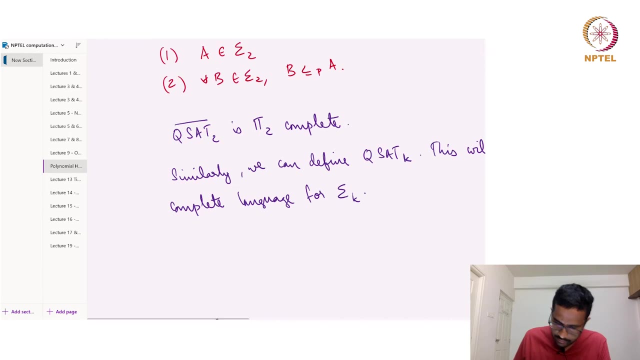 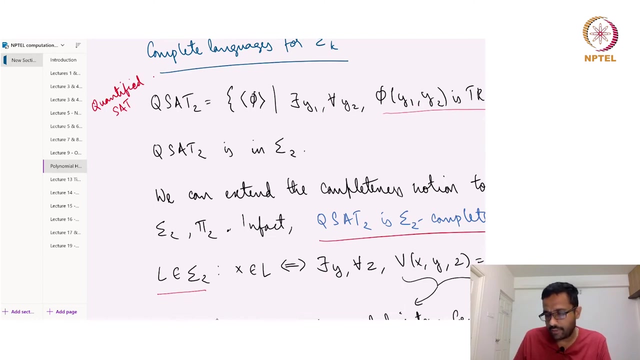 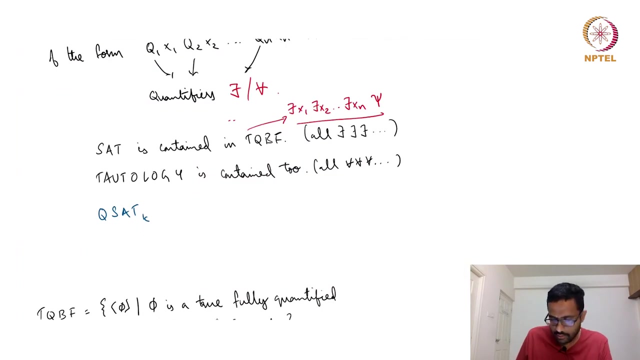 these languages called QSAT subscript k, right So they were, when we discussed a polynomial hierarchy, So this were of the form. so just to recollect, right, QSAT subscript k, So QSAT 2 was there exists y1 such that for all y2 the formula is true, right? So where y1? 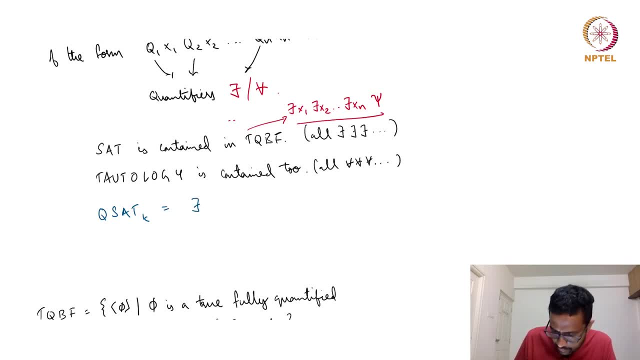 and y2 are sets of variables. So there exists y1, such that for all y2.. So these are sets of variables. Okay, Okay, Okay. So there exists some formula, psi of y1, y2, this is true, right? So even that QSAT sorry. 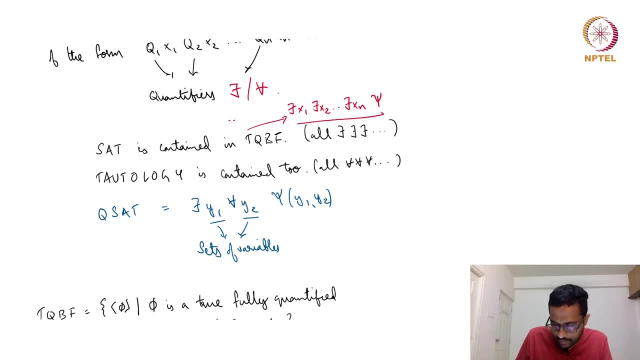 this is QSAT 2, but similarly you can write QSAT k, just that the number of alternations will increase, but then all the variables are quantified right. So y1 contains some variables. everything that is not there in y1 will be there in y2.. So QSAT 2 is in. 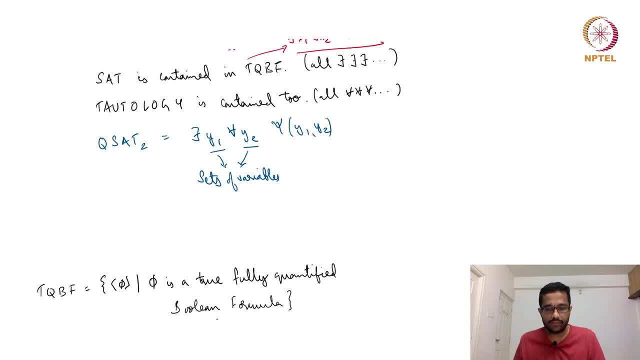 is quantified. So QSAT k can be written as a TQBF and hence, yeah, in anything QSAT k can also be contained in TQBF. So QSAT k, or even QSAT k complement, is contained in TQBF. They are all they can. 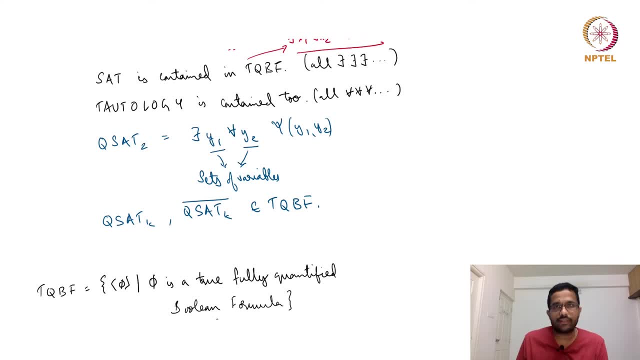 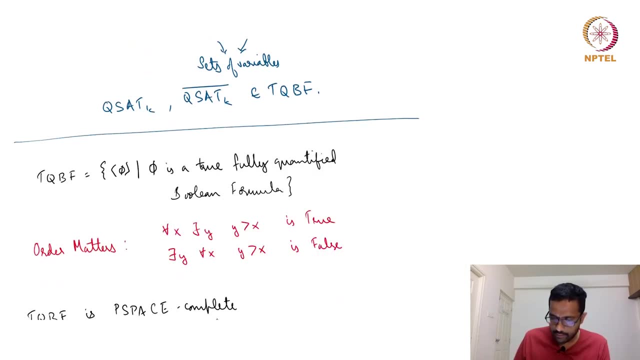 all be represented as fully quantified Boolean formula, which we are asking whether they are true or not. Okay, So yeah, formal definition phi is a true, fully quantified Boolean formula. but anyway, I have explained it And this, I have said this before, I will say it again. the order: 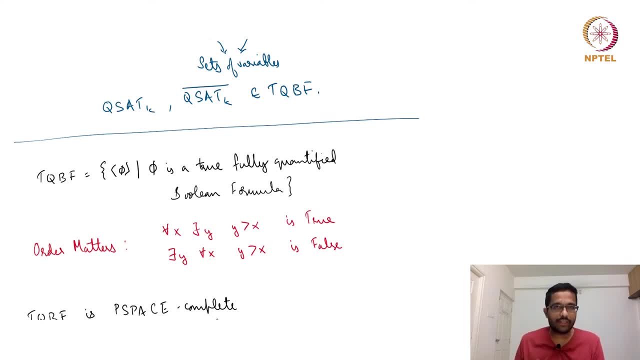 of the quantifiers matters. So it is not like if you swap the order or something else. the meaning is retained because of, let us say, integers. for all x does there exist a y, such that y is greater than x, where x and y come from integers? 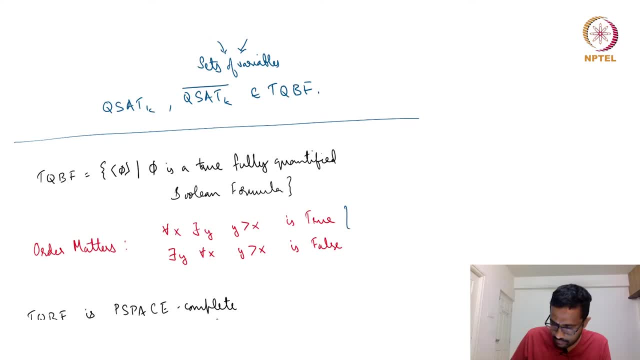 Okay, Where x, y are integers, There is no. so whatever integer x is, I could pick a y that is bigger than x. So the first one is true, But there is. if you swap the order it does not work. 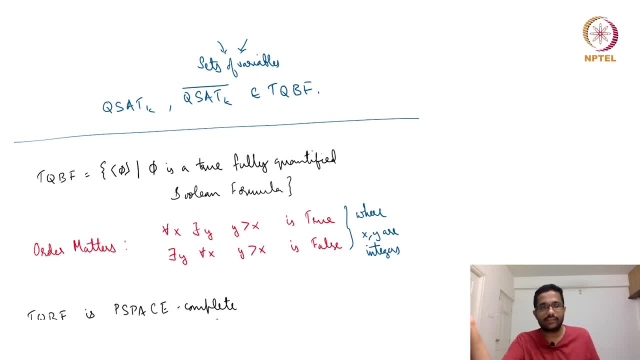 because there is no y that is bigger than all the other, all the x, So there is no integer that is bigger than all the other integers. If you tell me a specific integer, I can always produce an integer that is bigger than that, But there is no specific there. 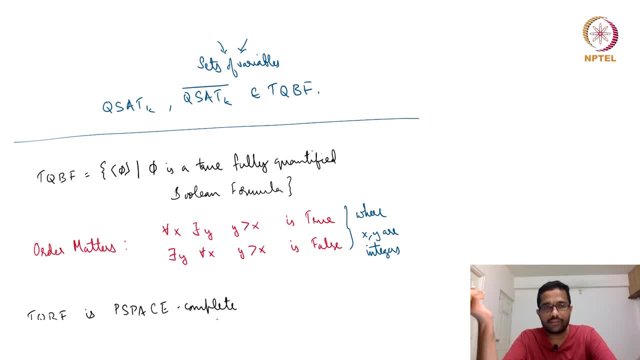 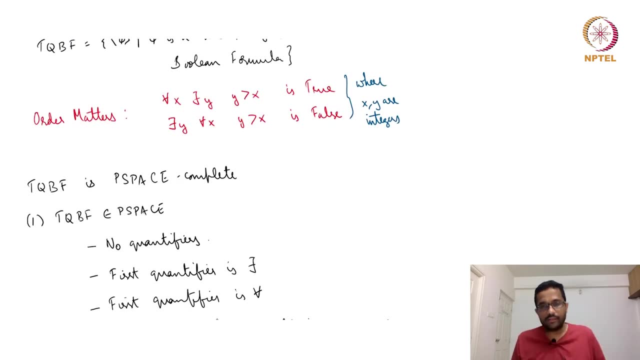 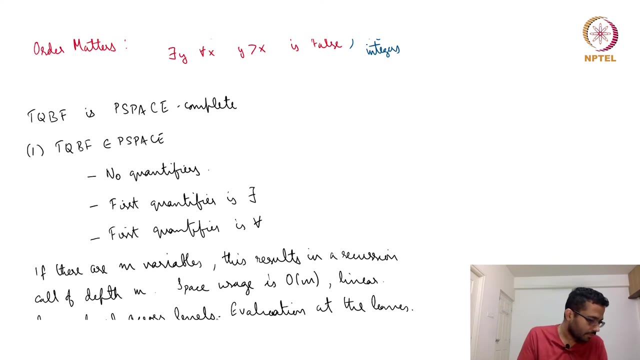 is no integer that is bigger than all the integers that you can give me. So the second one is false Again. this I have already explained. So TQBF is PSPACE complete. Why is this? So let us see why this is the case Again. why is this the case? 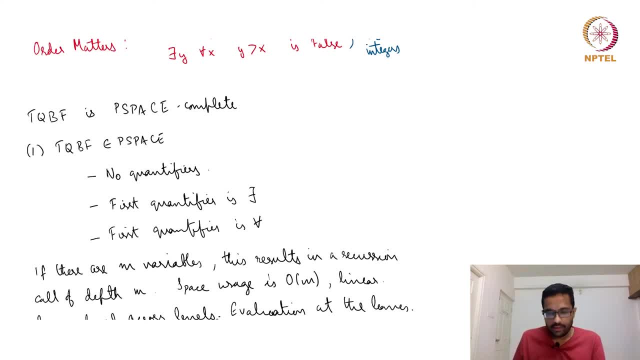 So there could be. what are the possibilities? So one is that there is no quantifiers, But TQBF means all the variables are quantified, which means if there are no quantifiers, there could be no variables. So this means it is a formula without any variables. So formula: 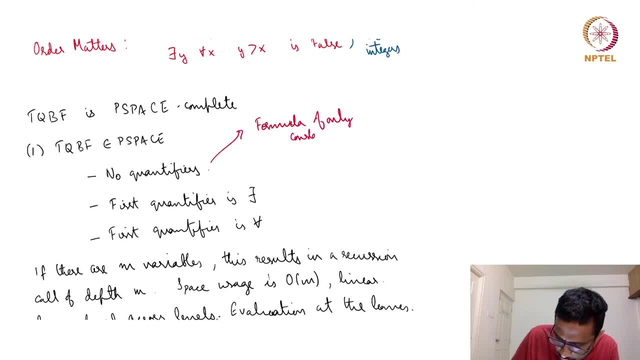 of only constants. So if it is a constant formula, it is something like the Boolean, like true or true and false or something like that. Just take a 3 plus 4 multiplied by 6, some numerical equation without variables. it is just like a Boolean equation without variables. 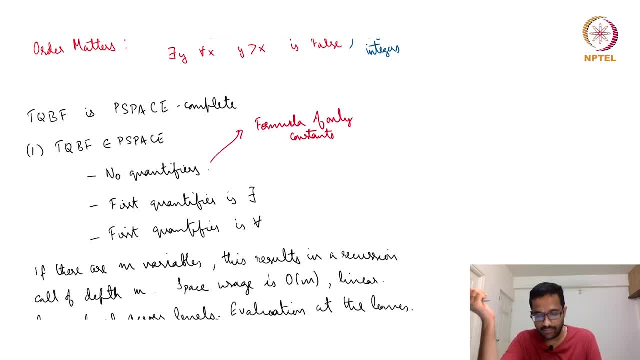 And one can easily evaluate that without much difficulty. So this is certainly in PSPACE. Now what if there are quantifiers? Let us look at the cases. So look at the first quantifier. There are two possibilities. The first quantifier is an existential quantifier that exists. 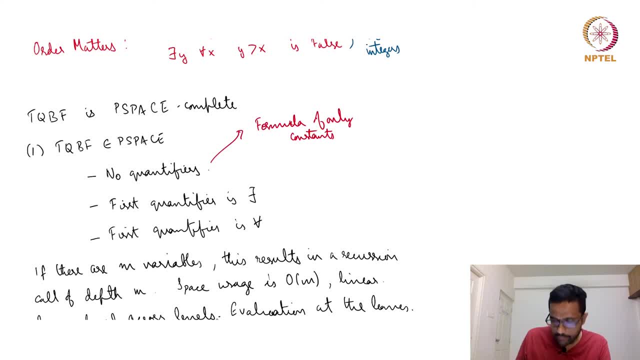 or an universal quantifier for all. So let us consider both. So let us say: the first quantifier is there exist quantifier, existential quantifier, So it says there exists x1 and something else, some, something else. So there could be other variables in this, something else. 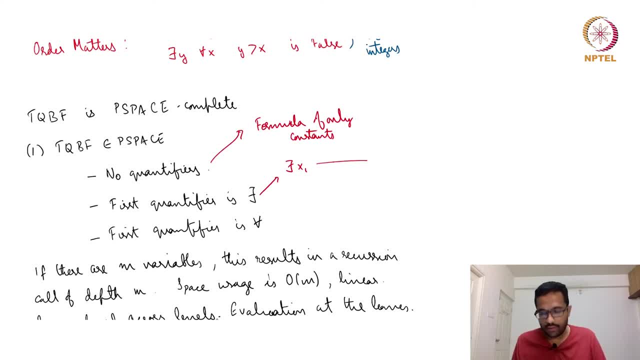 Now how do we solve this? So we want to check whether, so now the formula is saying so, some formula, this formula is saying so, this could be psi of x1, x2, something, something, something where the psi also contains quantifiers, or maybe let me just say phi of this, where phi also 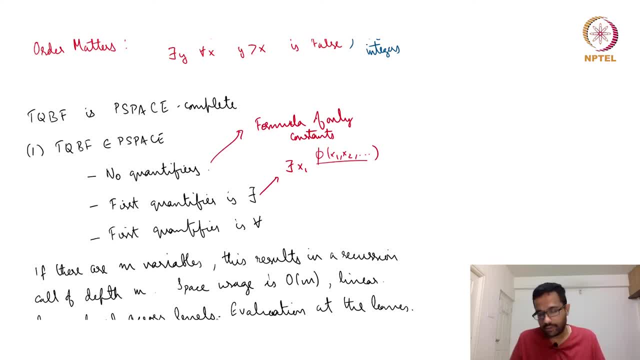 contains quantifiers. It will have quantifiers because so now we could set x1 to true and see whether phi is true, because it is true, So let us look at the second quantifier. So let us look at the second quantifier, because everything else is quantified inside phi except x1.. 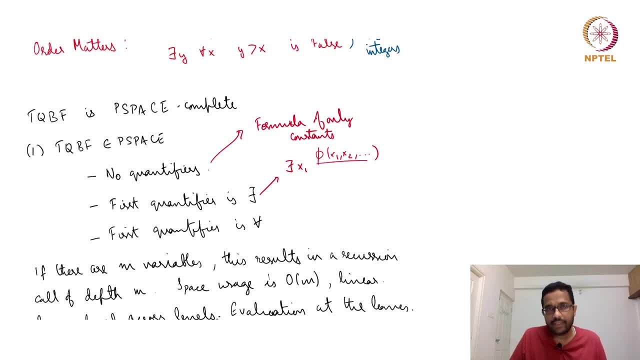 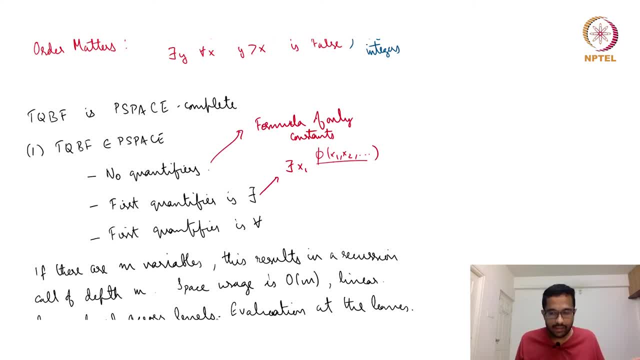 it is a TQBF instance And we want to check whether for. so the question is: does there exist an x1 such that phi is true? So you will check either: is phi x1, is phi true x2,, x3,, etcetera? 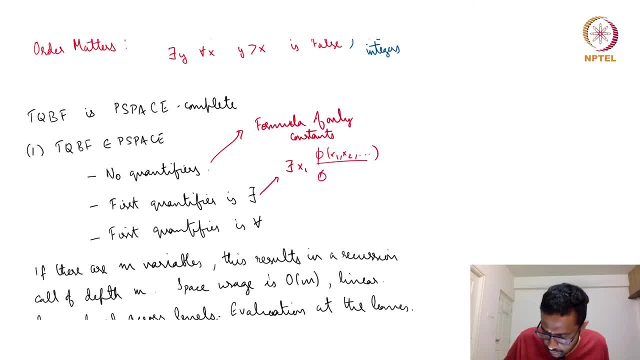 is that true or phi? so phi true, x2, etcetera. is this true or phi false? x2, etcetera. is one of these true because both of them are TQBF instances. Now, when the first? so again it is a recursive thing. The second thing is when the first. 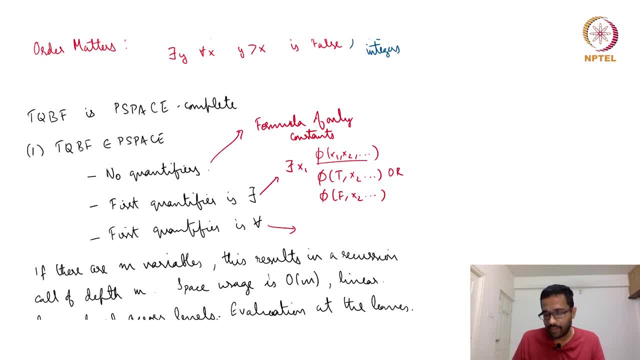 quantifier is a universal quantifier. again, it is not very difficult. You could think of it as for all x1 something, but it is exactly what I described for the universal existential quantifier, except that now we want both cases to be true. So we will check both branches and check. 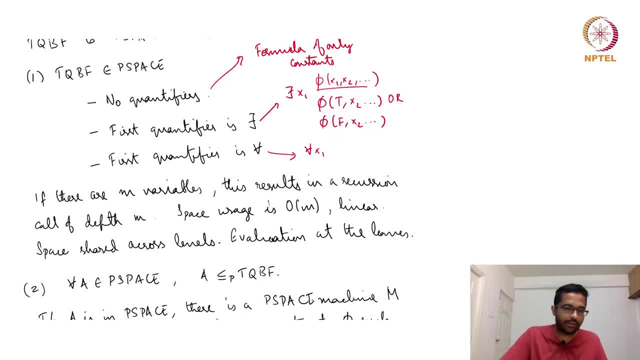 both of them are true. So what needs to be done here? It is a recursive call, So at each instance the tentative assignment of phi is x1 is stored, and then in the next level of recursion, x2 will be stored, and the next level of recursion, the next assignment of x3, will be stored, and so on. 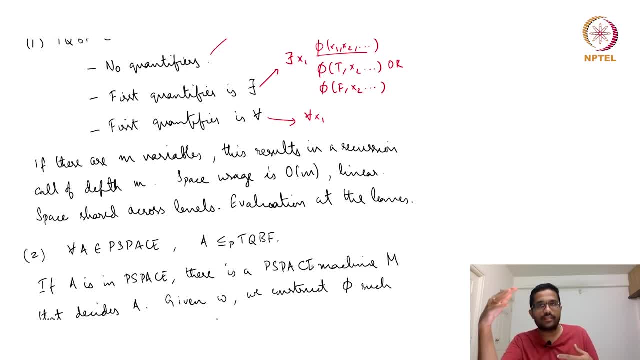 So if there are m variables, m variables in this fully quantified Boolean formula, we need to remember order m variables assignment. So that is order m: m bits are required. And then finally, at the end we will just make a. 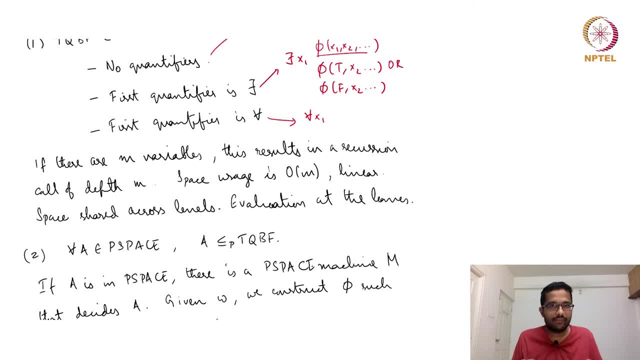 we will just try to evaluate whether this is true or not. So we will just have an equation of constants, a Boolean equation of constants which can be evaluated, And then at the end, all these branches have to be combined like existential means. there should 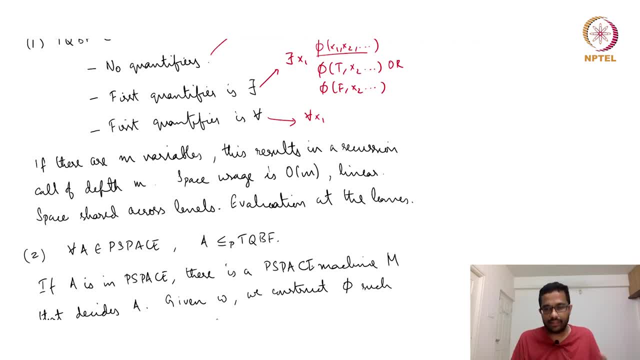 any one of the choices should be true. So all this can be done at the base, at the top level. So the space usage is order m, because there are mth items to be remembered at most. So again this. so this is the high level. 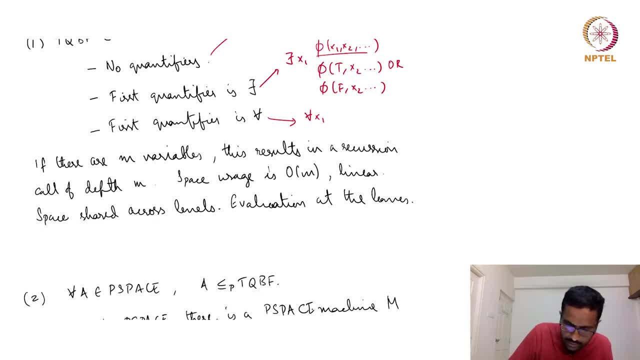 idea and this proof is there in Sipser. read full proof in Sipser. Anyway, I explained the full proof here. maybe I just did not write it down, but it is there in Sipser anyway. So this is the proof that TQBF is in V space. So the space usage is order m. 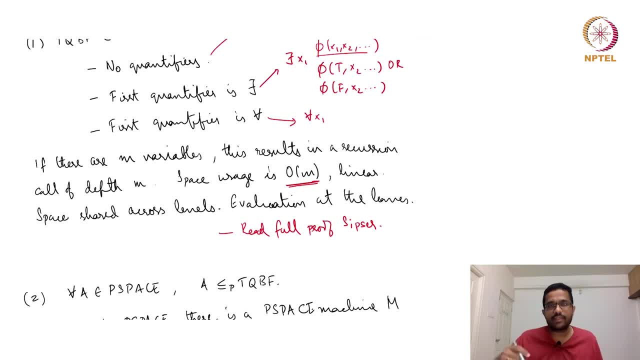 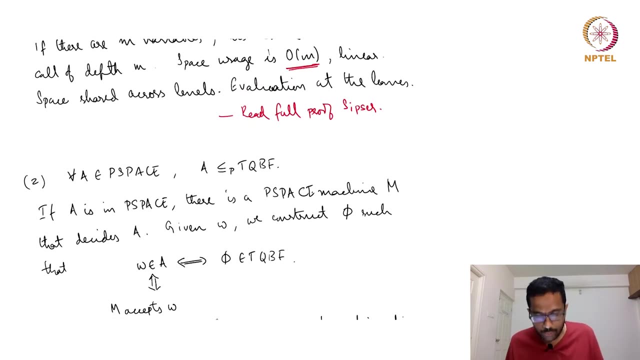 which is linear space. And this space is for all those recursion levels, not just one level, Because at each level a constant amount of space is required to store whether x1 is true or that kind of thing, true or false. Now let us come to the bigger question, which is whether it is P space hard. 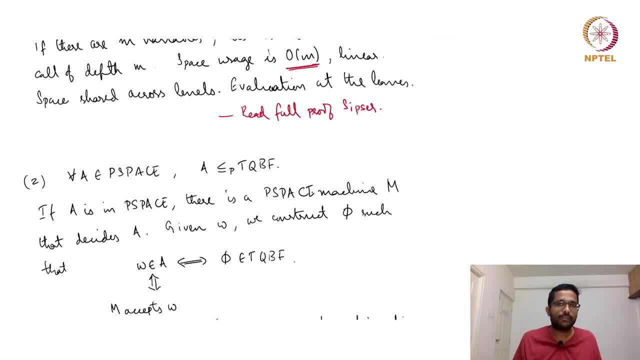 Like NP hard. we want to show that all the languages in P space are reducible to TQBF. For all a in P space, a should be reducible to TQBF. So it might help to recall some details of the Cook-Levin theorem proof. 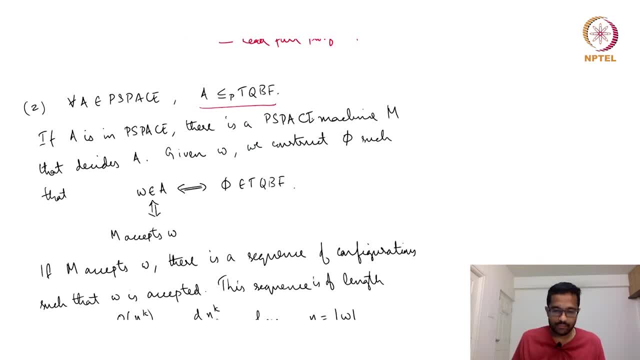 So if a is in P space, then. so this is going to be similar to that, but just that we would not go to the details because we have already seen the details in the Cook-Levin theorem, So we will just appeal to. 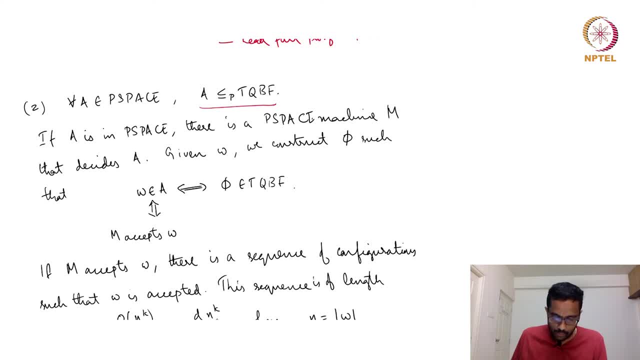 what we did then. If a is in P space, there is a P space machine that decides a. there is a P space deterministic machine. Now, given a string w, we can construct a formula such that w is in a if, and only if, that formula is in TQBF. 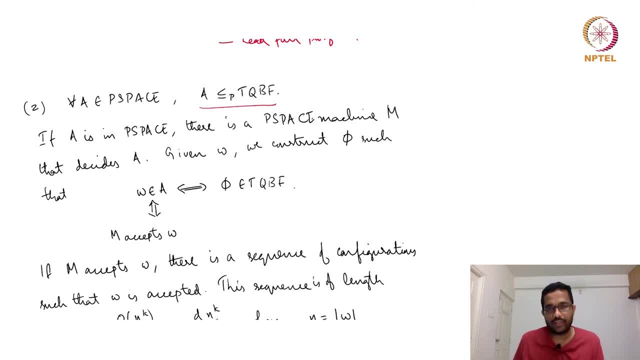 That is a high level idea of the proof. This is how we will do reductions. You want to show that, given a string, w is in a if, and only if, some fully quantified Boolean formula is in TQBF. This is what we want to show. So how do we try to show this? 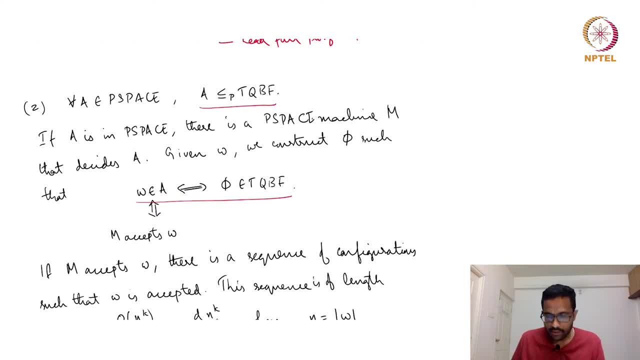 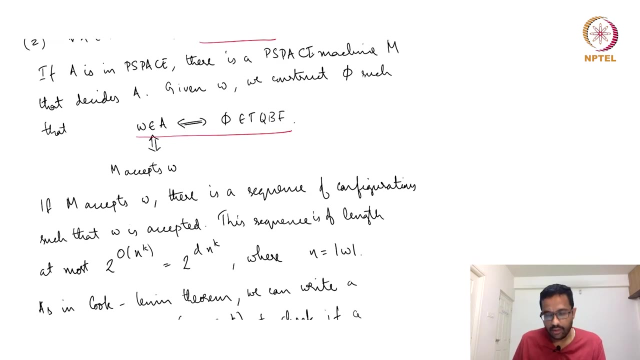 This is the goal of the reduction. The second point of the reduction is that the construction of the instance phi should be in polynomial space- sorry, polynomial time, because this is a polynomial time reduction. So the construction of this formula should be in polynomial time. So how does? how is that going? 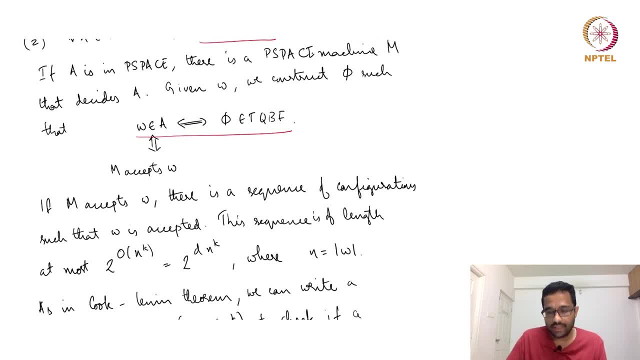 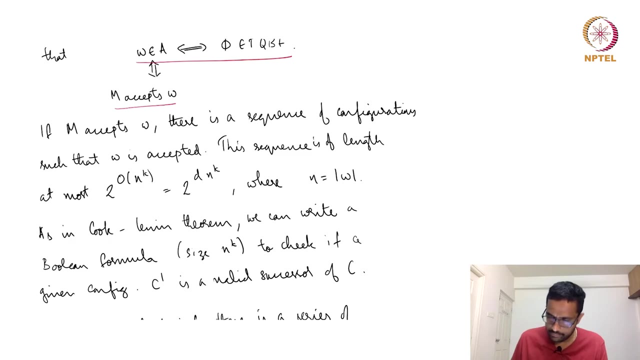 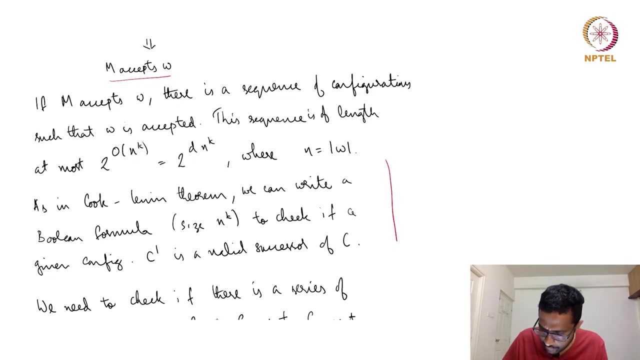 to work. So, as I already said, there is a PSPACE machine, M, that decides A. So W is in A if, and only if, M accepts W. So we will use M and W to construct this formula. So if M accepts W, that means there is a. there is a computation table that you can draw. 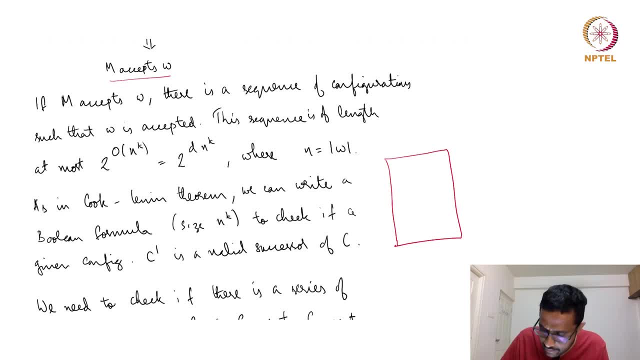 We know it is a polynomial space machine. Let us say the space, let us say it has single tape, let us say the tape usage is n power k. The tape usage is n power k And what is the number of? what is the? 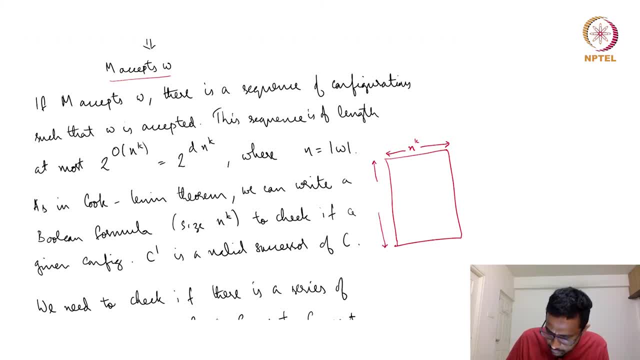 height of the table, This computation table. it is a maximum number of rows it can have. Each row corresponds to a configuration of the machine. How many configurations can we have before we start? If we see a same configuration again, it means we are looping, which means we are not. 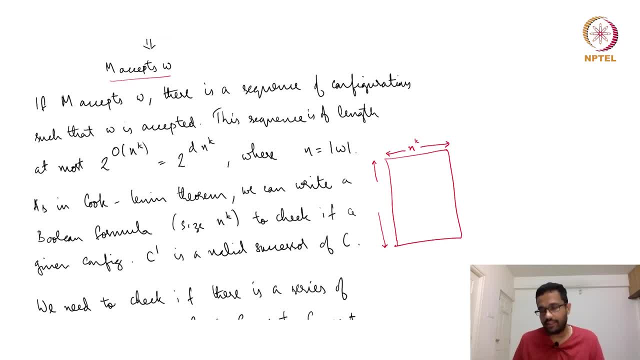 we have come to the same configuration again. Again, we will come back to the same thing and we are looping. So what is the maximum number of distinct configurations that you can see- And we have done this calculation many times- It is the maximum number of configurations that we can have. 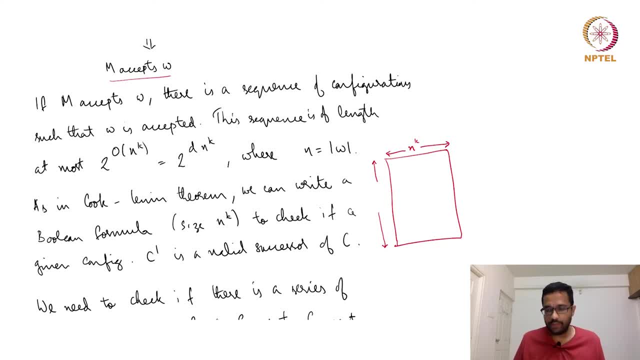 for a space bounded machine. So if we have an n power k space bounded machine, the number of configurations will be 2 power d n times n power k, where d is some constant and n is the length of the input. So this is like Kuklevin theorem, But in Kuklevin theorem it was time bounded. 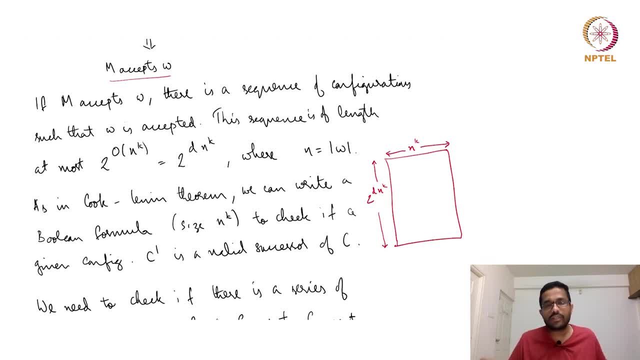 So the number of rows was n power k, and because the number of the time was n power k, we said that the columns also will be n power k, the space usage will be n power k. But here it works differently, because here we first know. 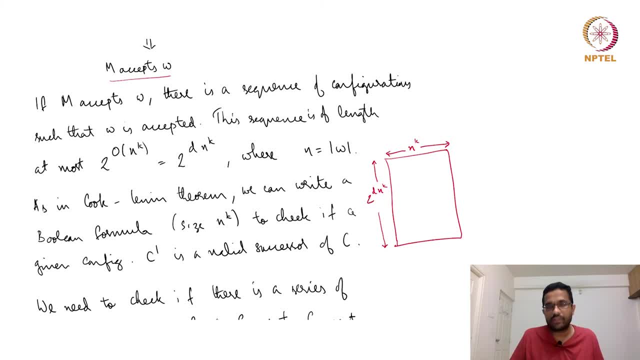 that the bound on the, we first know the bound on the number of columns or the space usage, And because of the columns are bounded. because the columns are bounded, the space is bounded. we know the bound of the configurations. hence the time of the computation will also be bounded. 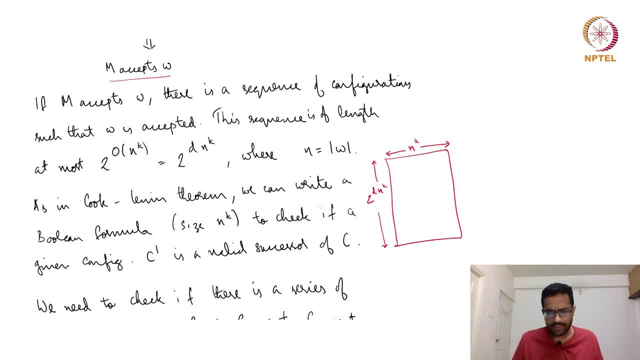 It will be exponential in in the space. Again, we have seen this. d time or d space f? n is contained in d time 2 power order f n. So it is the same thing here. Now again, this is a deterministic machine. 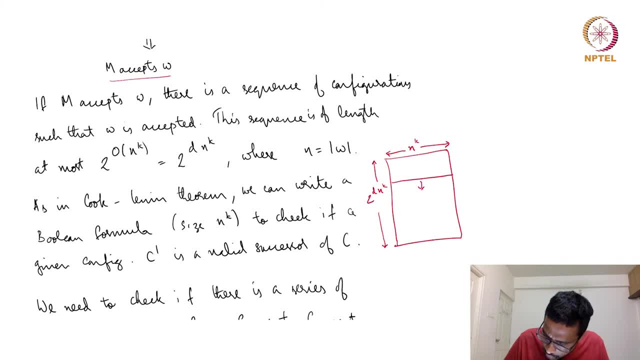 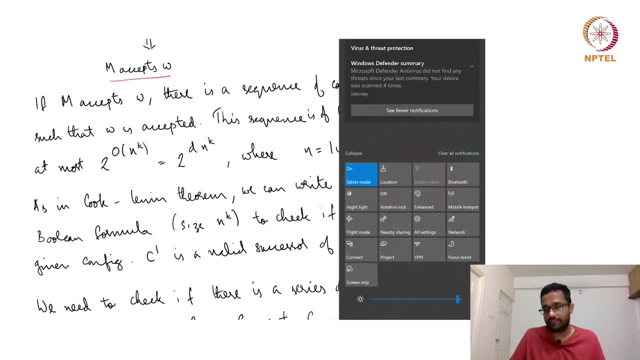 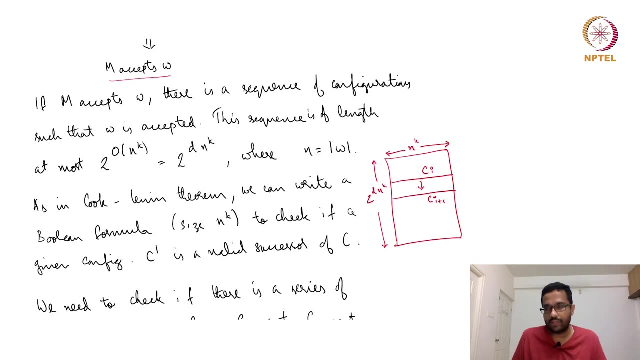 So, just like in Kuklevin theorem, we can write a formula, Boolean formula, to check whether c i or c i plus 1 is a proper successor of c i. sorry, A configuration i plus 1 is a successor of configuration i. We can write a Boolean formula for it. 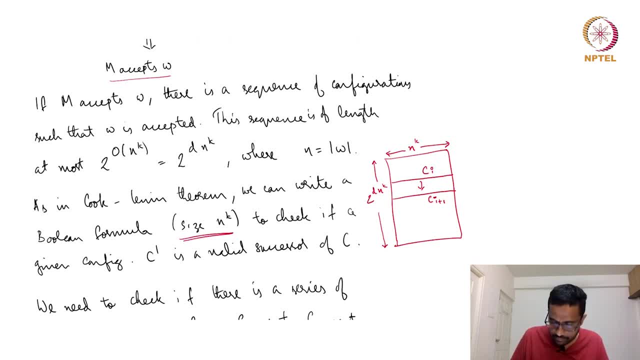 And this formula will be of size n, power k. So, given to check whether some configuration c c is, or maybe I will just make it more clear here- c i plus 1 is a valid configuration of c i. Okay, So basically we need to check. we know the condition of configuration i, but we also know that the configuration of c i is n to the power k n. so we stronger or better thought. So once again we will add a given value to our phul balloon. So we take a minor function of. we can write a scenario as follows: that Wi plus 1, n. 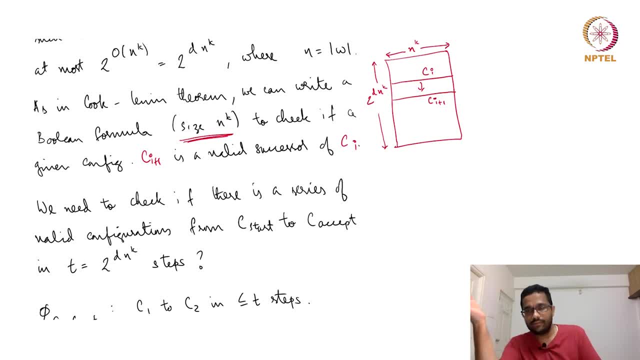 so Ц i plus 1 cannot be given or we punished it. So I do Ð to say c? i and I do Ð Jegqult to check. we know the start configuration given a particular input. it is known, We know. 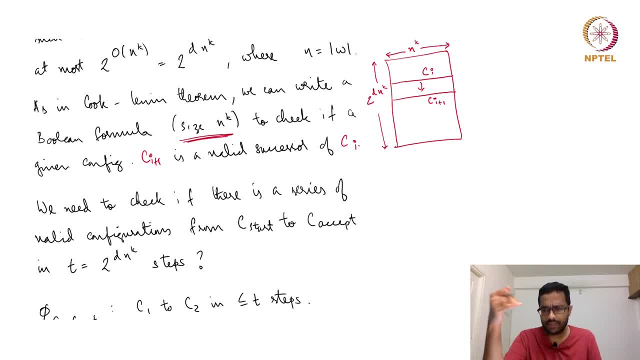 the accepting configuration. Again, we can do some things to make, we can force the machine to have a unique accepting configuration And we need to know whether there is a path from the start or path meaning a sequence of configuration from the start to the accepting. 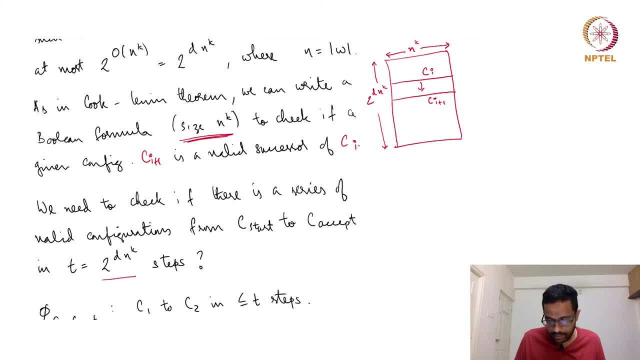 And we know that the maximum number of steps that we can have is 2 power d and power k steps. So can we, can this table, have a valid sequence of configurations such that the first is a starting configuration, last is accepting configuration and every configuration. 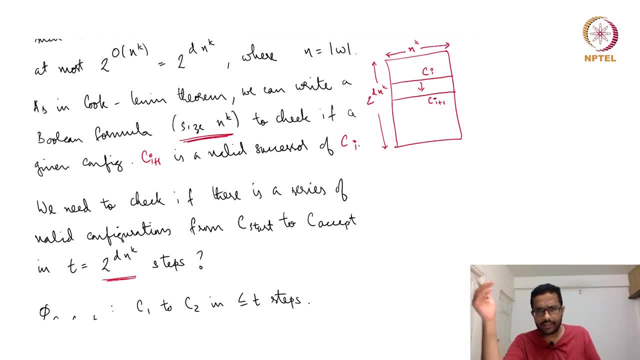 is a valid successor of the previous configuration. This is exactly what we did in Cook-Levin theorem. proof Just that in this case we are bothered about just that in this case one is that we have a deterministic machine, So presumably the number of successors are: 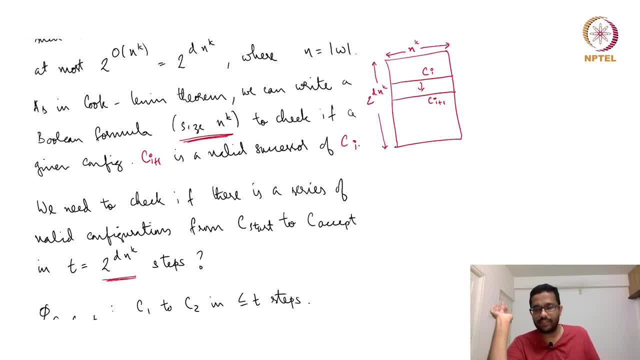 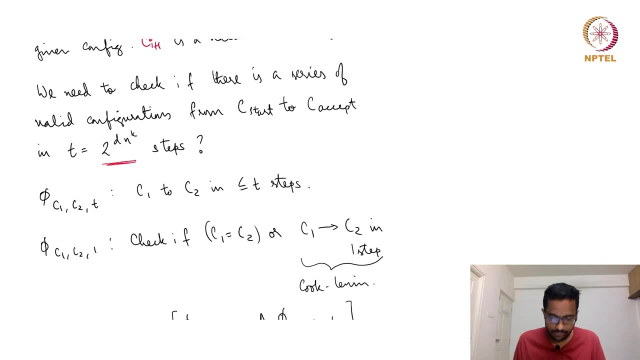 less, But that does not really feature in the computation anywhere. 2, the number of rows are higher. There we have n power k rows, here we have 2 power d times n power k rows, which is exponential in that. Now let us write a formula for this. So let phi c1, c2, t. So what we will do. 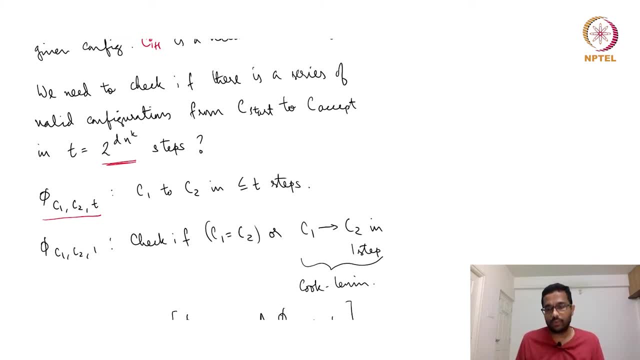 is, we will end up writing a fully quantified Boolean formula for this. So we will use all the quantifications and That we want. So the goal is to come up with something. Generally, we want to say: does there exist a sequence of configurations that takes you from c1 to c2 in t steps? So now, 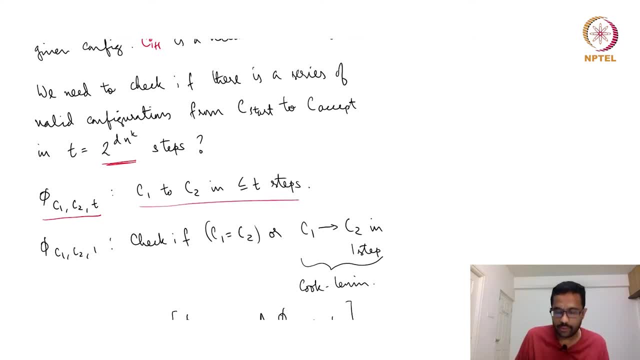 if we can accomplish this, then we can set c1 to c start, c2 to c accept and t to 2, power d times n, power k, So then we can solve whatever we want. So let us see what is c1,, c2, 1. Can we move from c1 to c2 in one step at most? c1,. 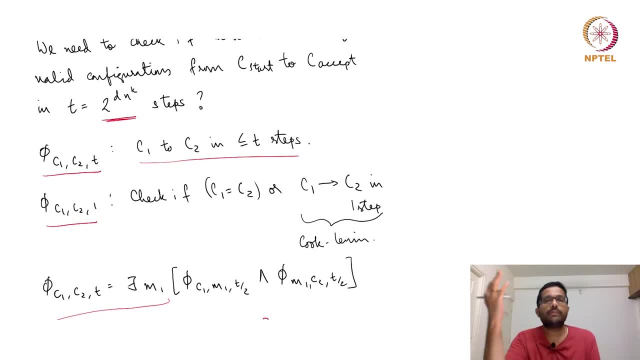 c2, 1.. So how can? what do you mean by one step? at most, Either the c1 and c2 are the same, which means 0 steps, or c1 and 1 step computation gives you c2.. So either c1, equal. 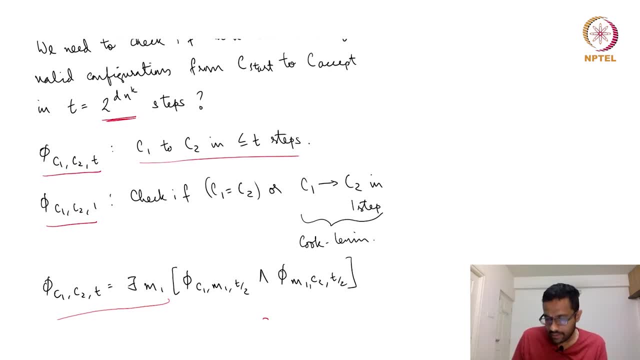 to c2 or c1 to c2 in one step, And this is not that difficult to do, because c1 equality can be easily checked And c1 to c2 in one step. again, it can be checked by what we saw in the proof of Cook-Levin. 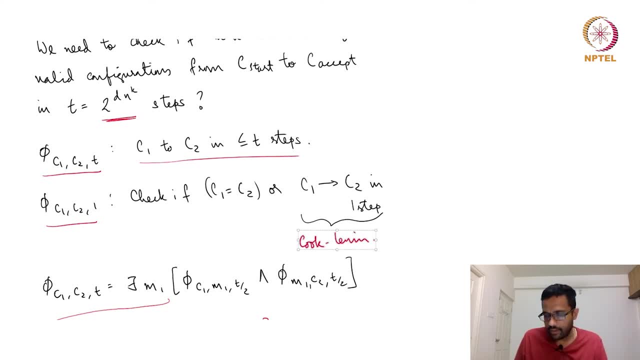 theorem. We had this phi move which was essentially this: this making windows into tables, and so on. So both of this can be done, So that is fine. So this formula is of size, I think, n power k Or order n power k, this entire thing. So that is good. Now we want to see whether 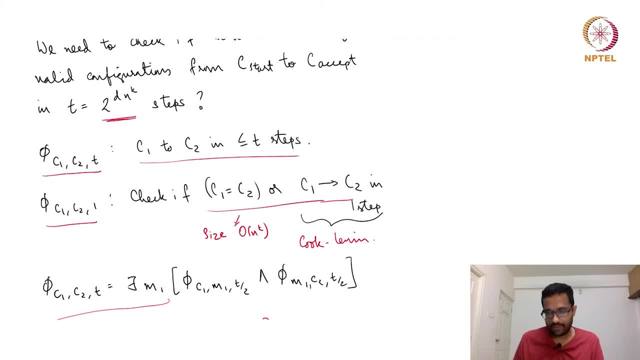 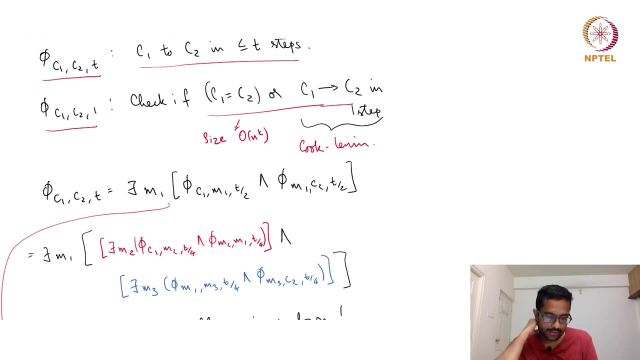 we can generalize this for not one step but t steps. So let us see again. we saw Savitch's theorem. Let us see how to write this in t steps. Because if you write in t steps one possible like, if you do it in like in Cook-Levin theorem, we will have to write c1, c2,, 1, c2,. 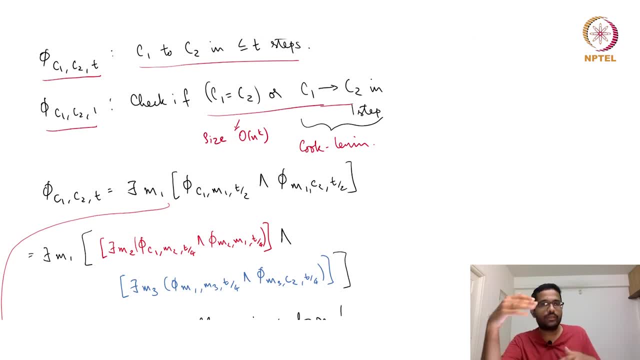 4 is successor of c3, c3 and so on, which will mean an exponential sequence of such things. So which is 2 power d times n power k times n power k, which will be? So we cannot afford to do this twice. 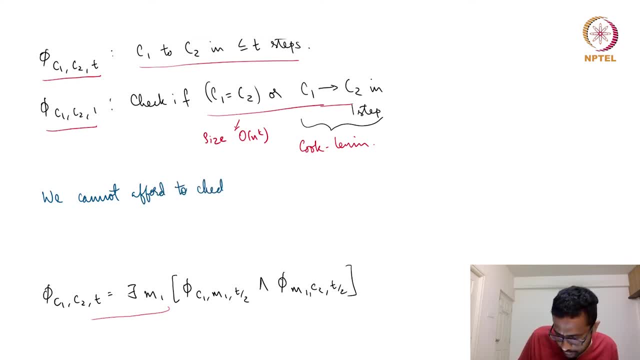 Ok, Ok, to check phi c1, c2, 1 and phi c2, c3, 1 and c3, c4, 1 and so on, because this will be exponential size. So we cannot afford to do that. So we cannot do that. So how do? 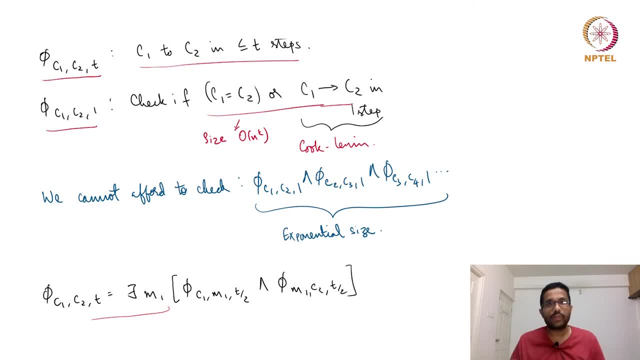 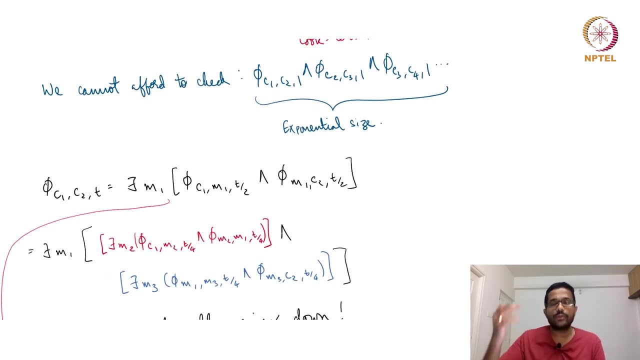 we do this more intelligently. We want to reduce the size of this formula. So what we will try to do is something that we tried in Savitch's theorem already: we will use recursion. So if there is a weight from c1 to c2 in t steps, then there should be a middle. 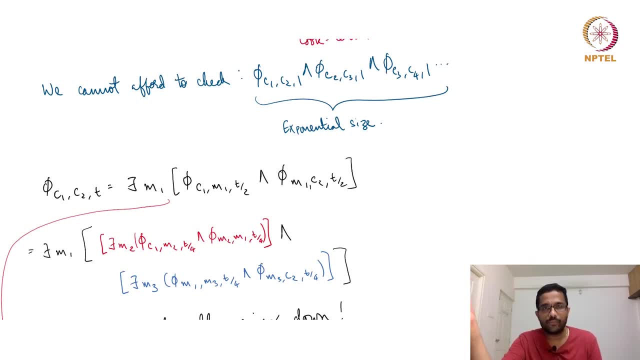 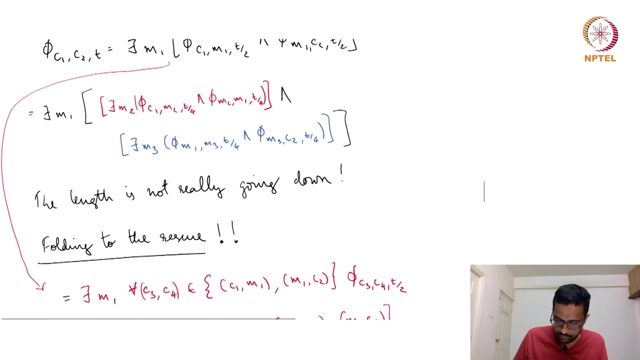 point at t by 2 steps, t over 2 steps. where were you? Let us say you were in some intermediate configuration called M1, so we do not even know what M1 is, but there may be some t over called M1. So I could write: does there exist an M1, such that from C1 to M1, you can go? 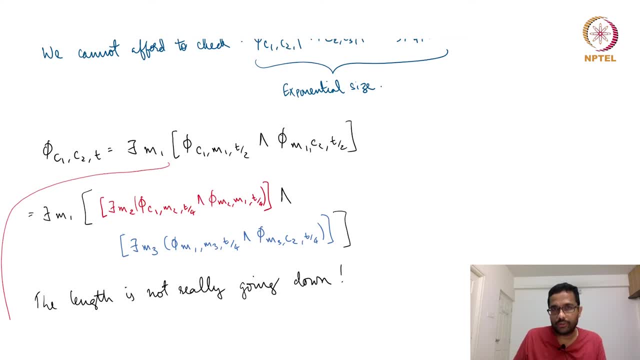 in T by 2 steps and M1 to C2, you can go in T over 2 steps, C1 to M1 in T over 2 and M1 to C2 in T over 2.. So basically this is the midpoint of the table. So C1 here, C2 here. 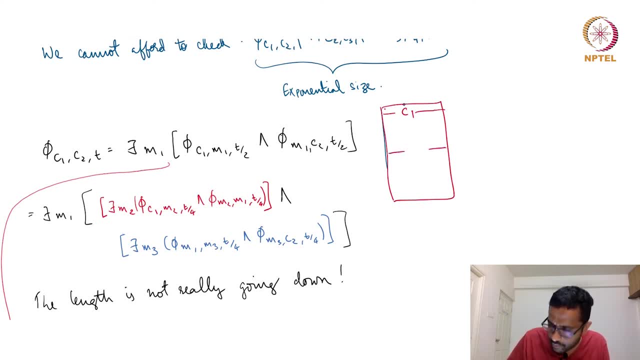 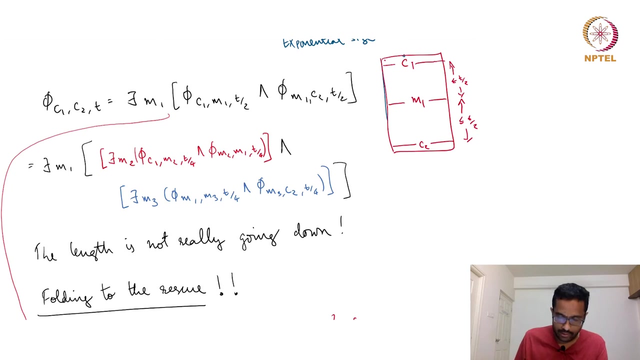 M1 here, which is roughly at the midpoint, So small M1 and C2 here. So this. so if you can go from C1 to C2 in at most T steps, then this should be possible. So now let us see what can be done. 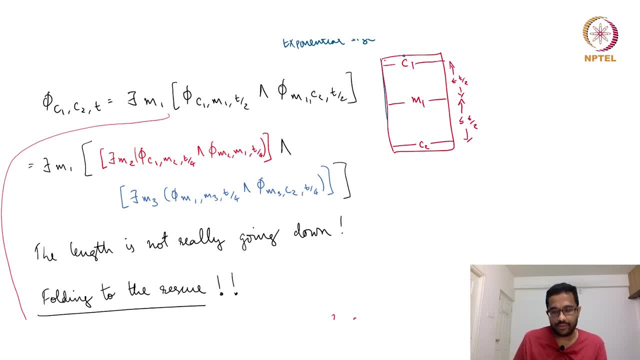 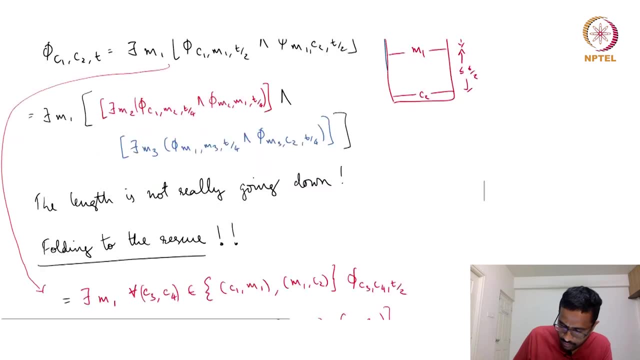 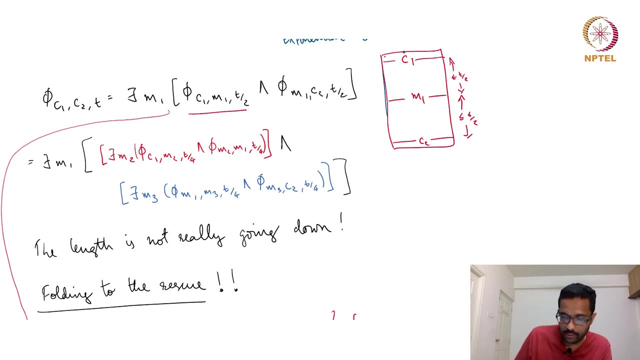 So now we could possibly repeat this trick again. So there exists M1, such that this is true. Now I could possibly rewrite, I could possibly rewrite this part C1- M1- T over 2 into in a similar fashion by this red color stuff, and M1- C2- T by 2 into this blue colored notation. So this here: 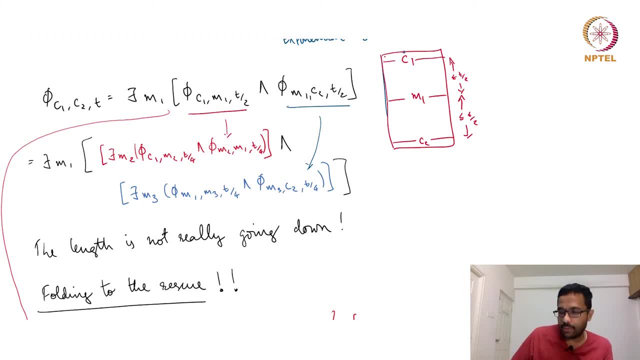 and this here, Basically, between C1 and M1, there has to be an intermediate notation. So this is the intermediate notation, So this is the intermediate notation, So this is M2. and between M1 and C2, there has to be an intermediate M3.. So we are checking whether 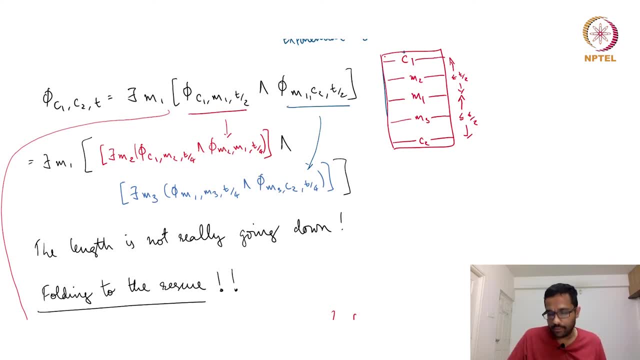 C1 to M2 can be traversed in T by 4, M2 to M1 can be traversed in T by 4, M1 to M3: T by 4, and M3 to C2- T by 4.. That gives you this kind of formula, But notice what is happening here. I have split. 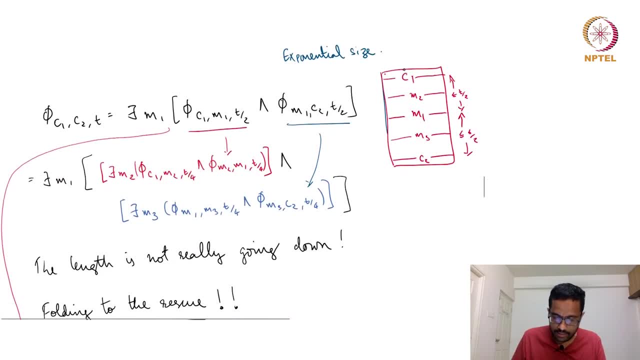 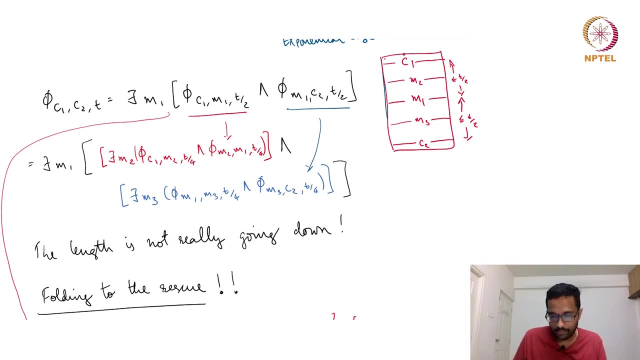 the original C1, C2, T into 4.. So we have 4 parts: C1, M2, M2, M1, M3, M1, M3, and so on, and the T became T divided by 4, and it is So now. 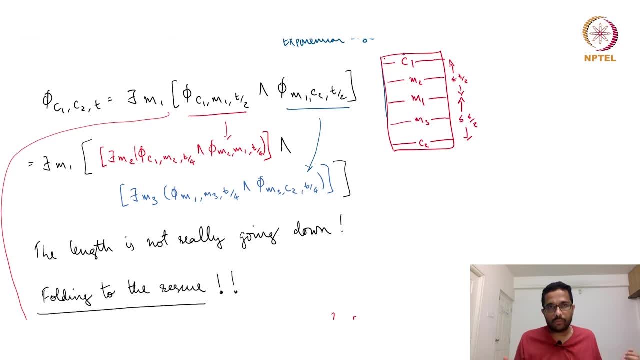 the T became one fourth and we have 4 parts. But now this is expanding and expanding and now this does not seem to be, and I think, even if we try to unroll this T by 4 into single steps, this will be actually the original situation. again, We will have an exponential sized formula without any 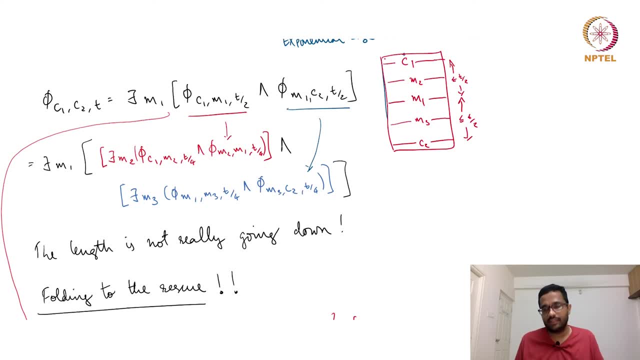 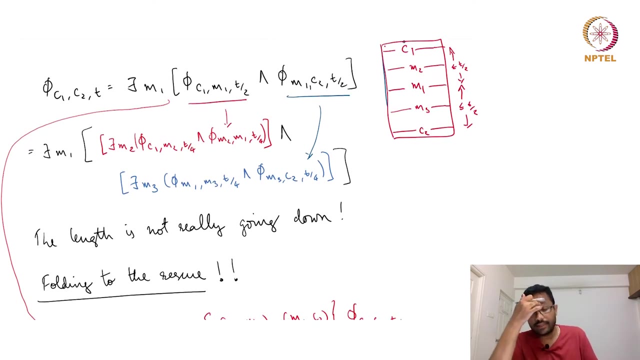 size reduction. So this is not going to help. This is just some. I am just using recursion but not really making progress here. So the length is not decreasing here. So now? so this is whatever we had in Savitch's theorem. does not really help, but we now use a new trick called folding. 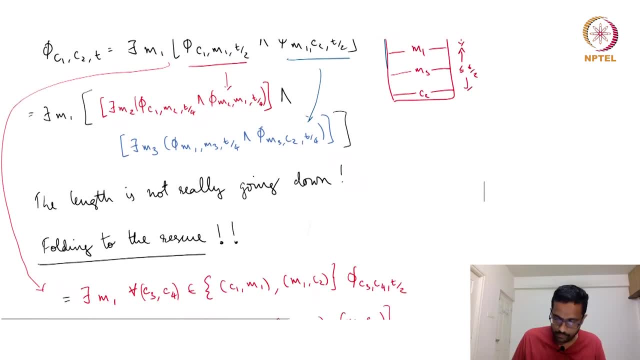 So what does folding mean? We will see now. So consider the. consider this top formula again. There exists M1, such that phi is C1- M1- T by 2, and M2 is C1- M1- T by 2.. So we have: 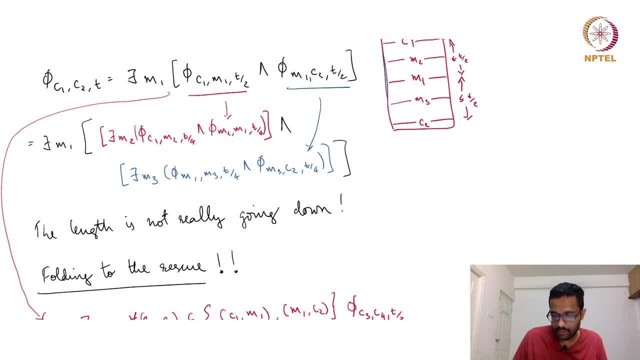 written down the variable same thing. just keep at M1 by 2 and phi M1 C by 2, T by 2, you are going to, we are going to1 C 1, T by 2, phi M 1 C, 2, T by 2, I am going to write the. 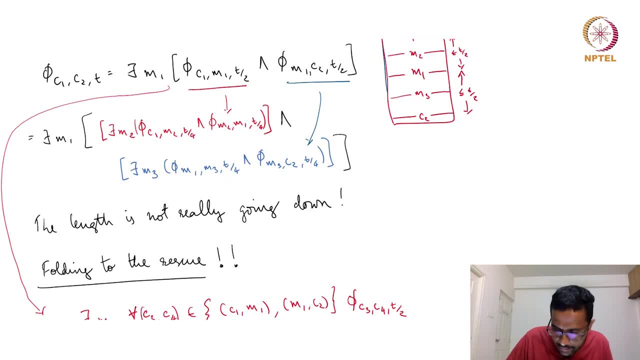 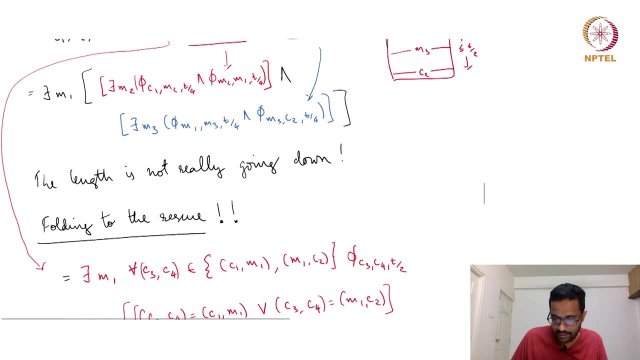 FO rule first in a new way. So instead of writing phi C 1 M1 T divided by 2 and phi M1 C 2 T divided by 2, I will just write it as So there exists M1 here, there exists. 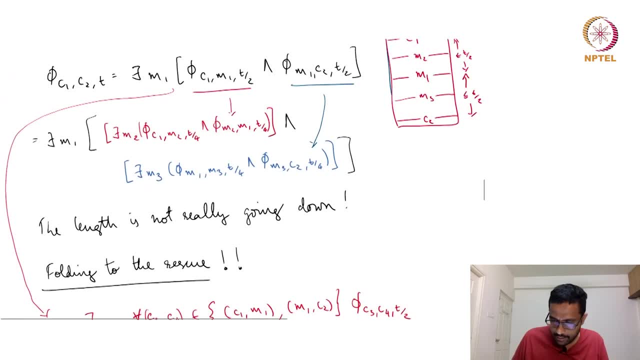 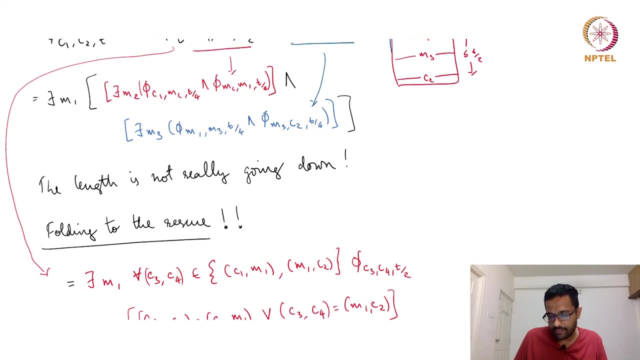 M1, same thing. I will write it as C 1, M1 and M 1, C 2 are the two points And then I two pairs. So I will let I will define new two variables: c3 and c4.. Whenever c3, c4 are, 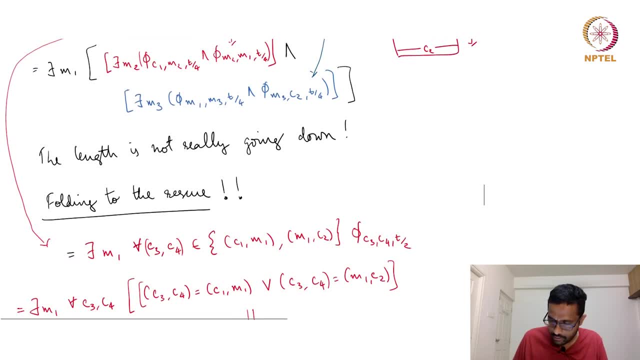 equal to sorry, c1, m1 and m1, c2, I will check phi c3, c4, t by 2.. Whenever c3, c4 are c1, m1 and m1, c2, I will check phi c3, c4, t by 2.. So when c3, c4 is c1, m1, I am. 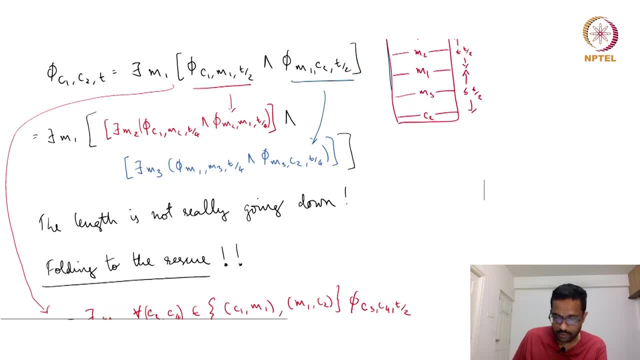 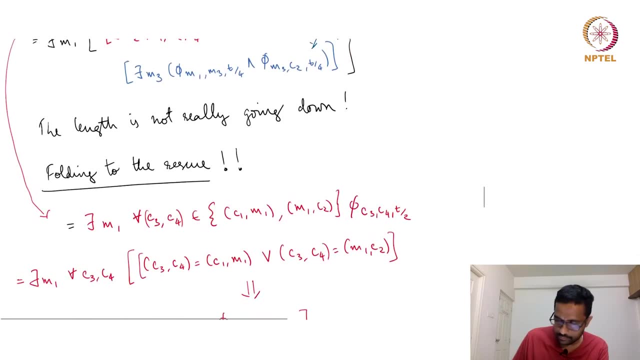 checking phi, c1, m1, t by 2, which is what we have. the first term here In c3, c4 is m1, c2, I am checking phi, m1, c2, t by 2.. So for all c3 and c4, such that they are like: 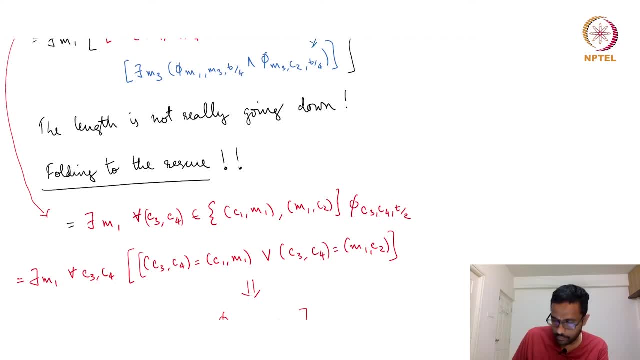 this. they are in c1, m1 or m1, c2, I do this, So I am using: there exists in M1 and for all C3, C4 in this set, So now I am using some new kind. 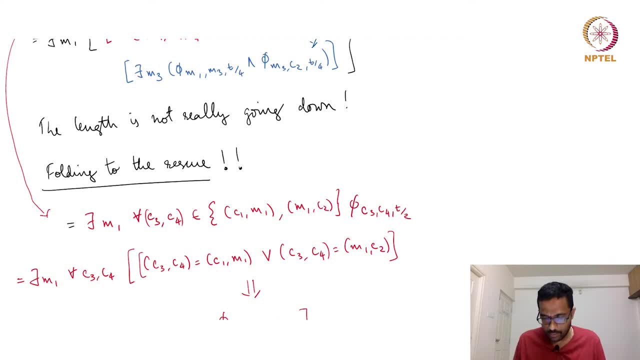 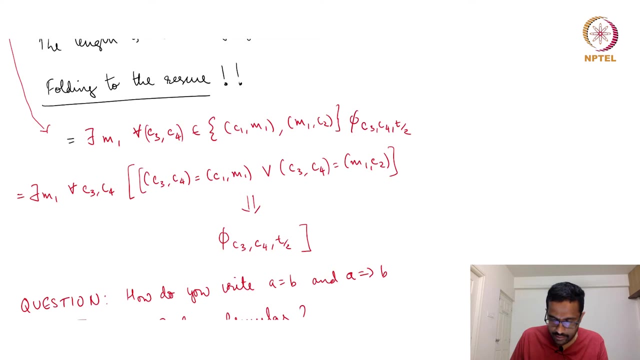 of expressions here. So I am using contains: is a member of C1, C1, M1.. How do we write that in a Boolean setting? It is not very difficult. So what you do is you can have a this particular part. this blue underlined part can be written by this part. sorry, can? 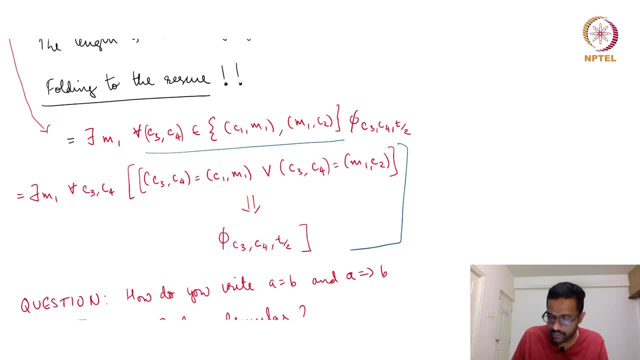 be rewritten by this entire thing. So whenever C3, C4 equal to C1, M1 or C3- C4 is equal to M1- C2, so this is M1- C2.. This kind of looks like an e, but it is C2.. 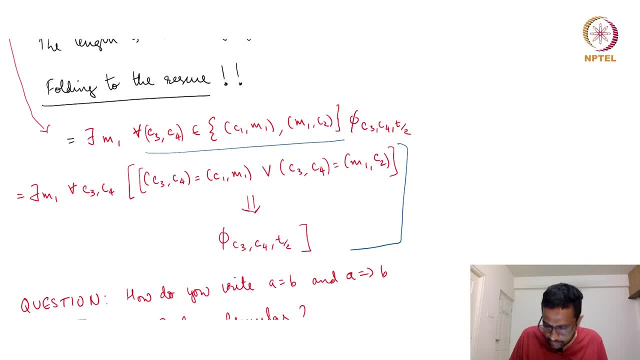 When this happens, this implies that phi, c3, c4, t2,, t divided by 2 must be true, So the rest is same phi m1 for all c3, c4, whenever c3- c4 is equal to c1 m1 or c3- c4 is m1- c2,. 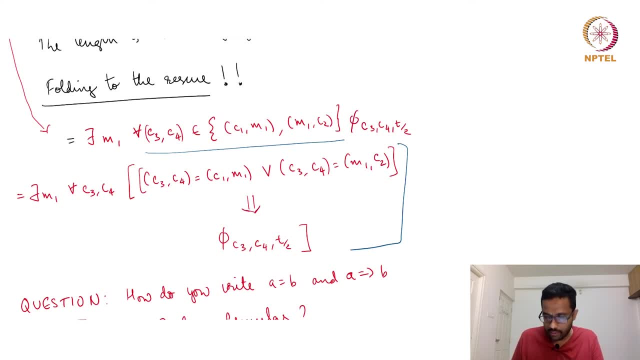 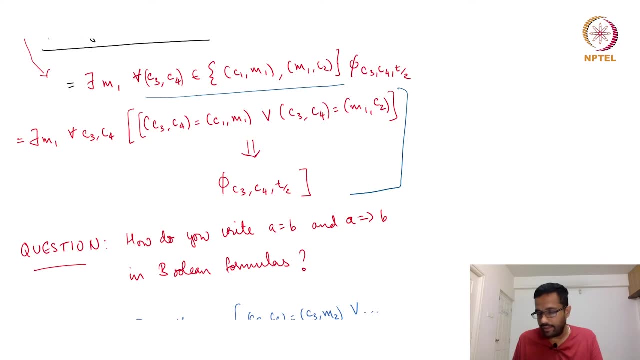 phi, c3, c4, t by 2.. So now, the first part is now. the only thing that is remaining is the equal to symbol and the implies symbol. Now, finally, I will leave it to you to think how to write- sorry, how to write the equal to symbol and the implies, a, implies b and a equal. 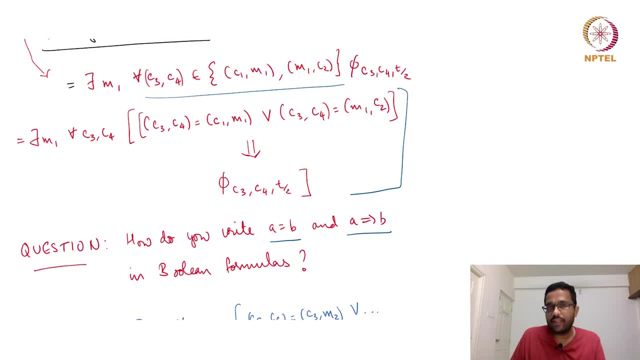 to b. how do you write it in a in a using just Boolean formulas? These are very, very simple exercises. Maybe you might have seen this in the first class in Boolean logic, So you can think about it. This is not very difficult. 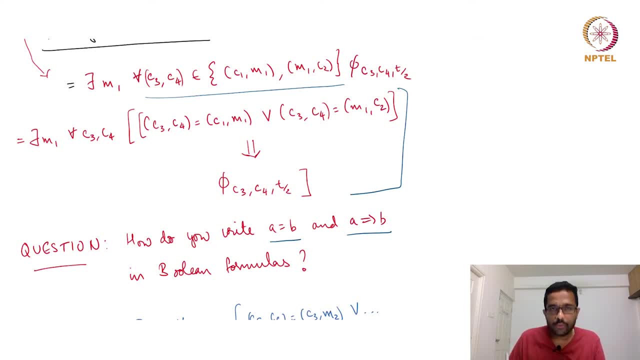 So you can. the point I want to impress upon you is that all this can be done in, all this can be done in using Boolean formulas. So now the formula is something like this: So this is this entire formula is now some constant multiplied by n, power k. 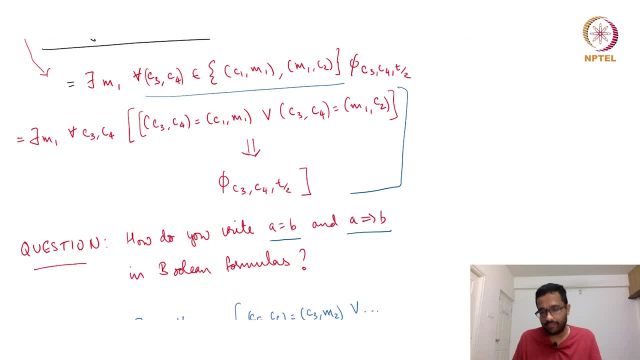 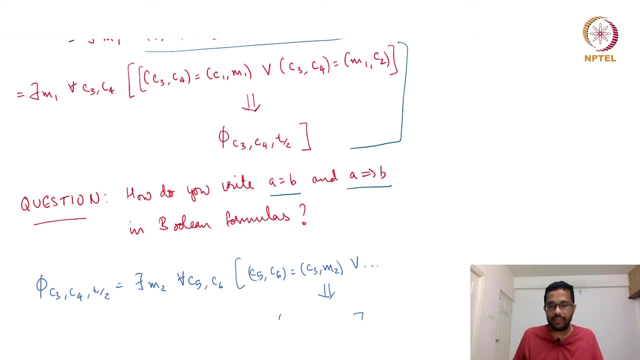 the part after the quantifiers. Now again, phi, c3, c4, t by 2 is a- is something that we need to go deeper into. So, phi, how do we go deeper into that? Again, we will use exactly the same thing. I can define intermediate. 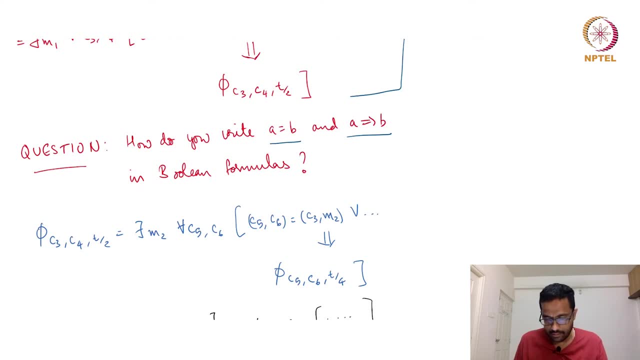 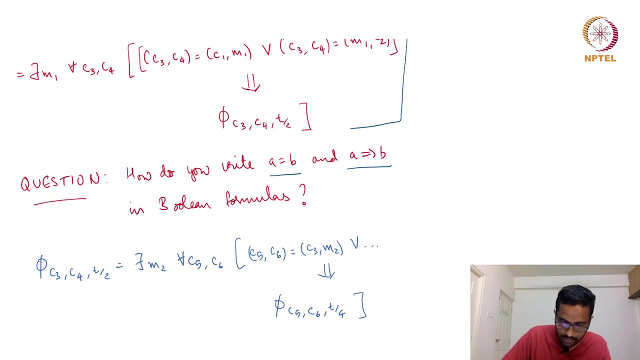 state c5 and c6, and the intermediate state, m2, and then variable c5 and c6, such that maybe I will just write it a bit- c5- c6 is equal to c3- m2.. Or c5- c6 is equal to m2,- sorry, sorry- is equal to m2- c4.. And when that happens, this: 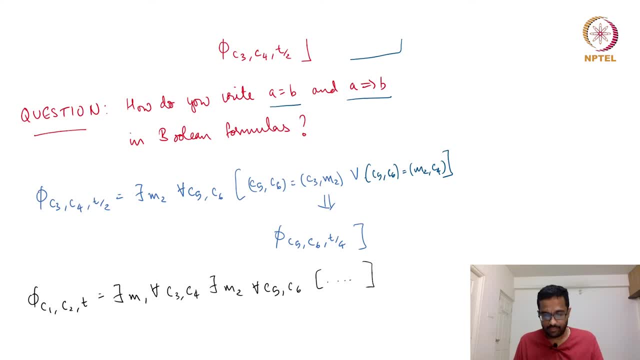 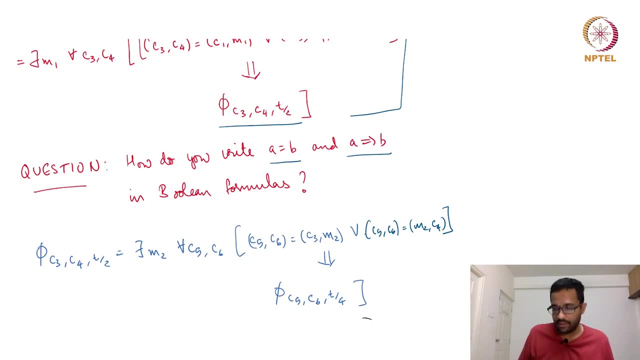 implies phi c5, c6, t divided by 4.. So this is how you expand out this quantity, the blue underlined quantity- phi c3, c4, t divided by 2.. So now, when I combine all this- so recall we were trying to write a formula for phi- 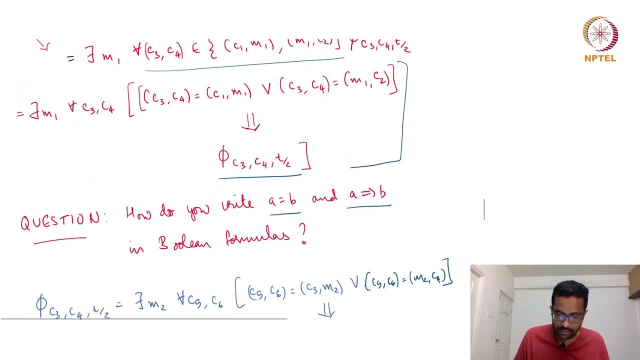 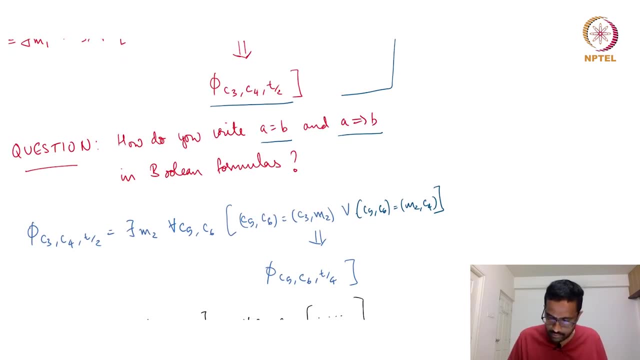 c1, c2, t, which we first wrote this as phi. there exists m1 such that for all c3, c4, something and the rest. So I can write it as: there exists m1 such that for all c3, c4, there exists. 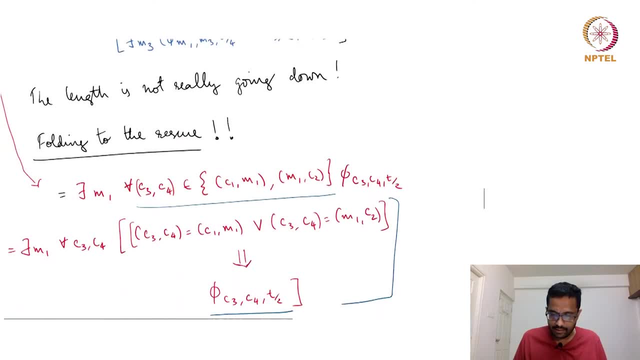 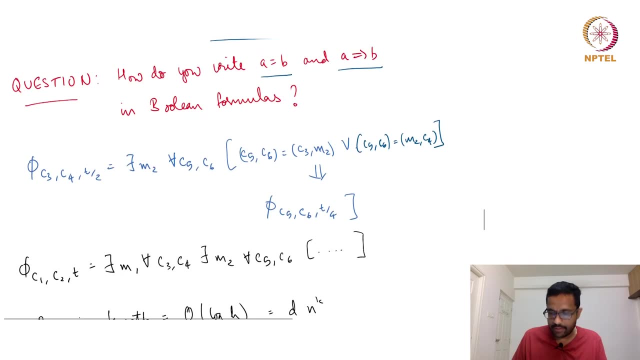 m2, such that there are for all c5, c6.. There will be some, some formulas involving c3, c4,, m1, all this and c5, c6, c3, all this, and then, finally, we will have phi, c5, c6, t by 4 as part. 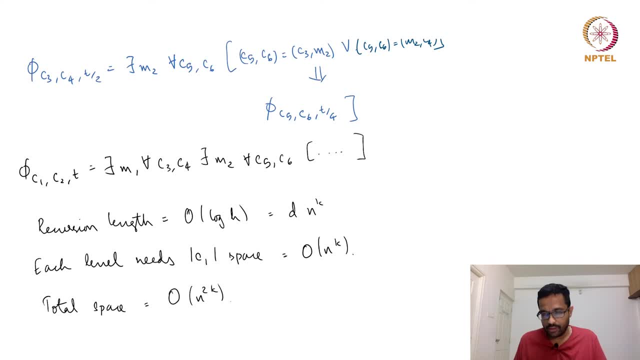 of this, which again can we go deeper and deeper into. So the point is that each level adds only a linear, some constant multiplied by n, power, k, which is each. this is what I have written here in the part that I am underlying now. 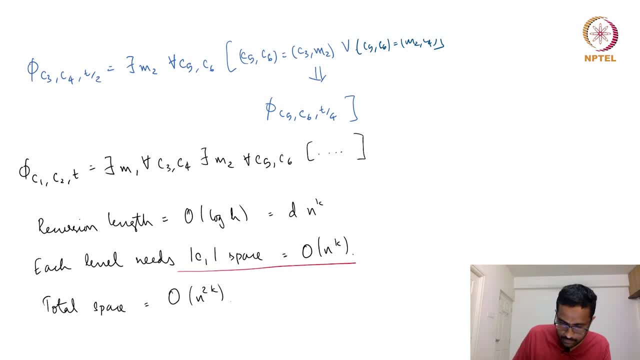 Each level needs extra spaces, some constant times order. So order size of C means order size of a configuration space And we know the size of a configuration is order n power k. So it is still another constant, so it is still. 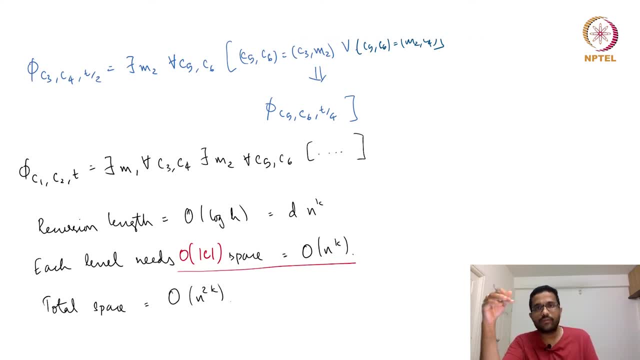 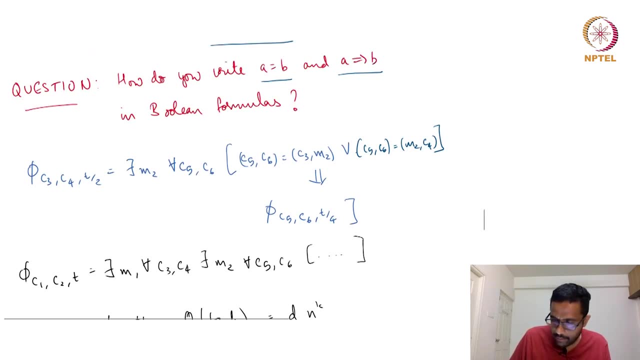 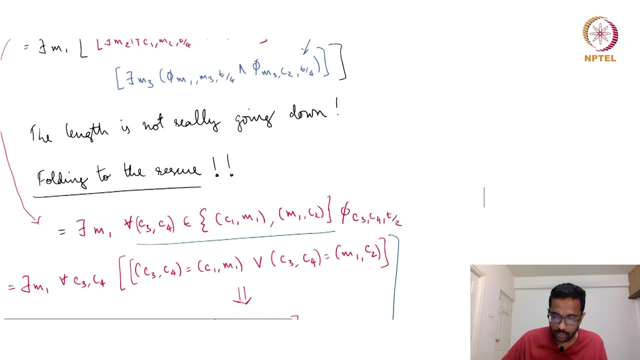 order n, power k: This is the extent of memory required at each level, And at each level, notice that the t became t by 2 and then t by 4.. So this, so every level, the t is halving And we know what to do at the base case when t equal to 1.. This is what we could do, This 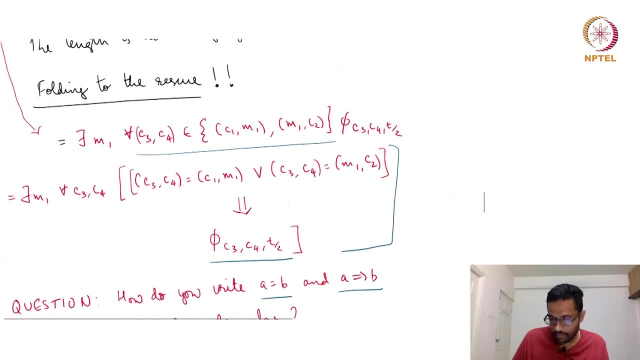 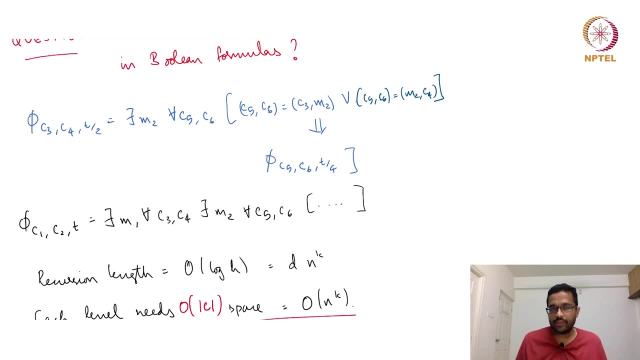 is what we did, So the base case is at 1.. So how many levels are required to go from t to t divided by 2 to t divided by 4?? So it is log t, number of levels, So, or the number. 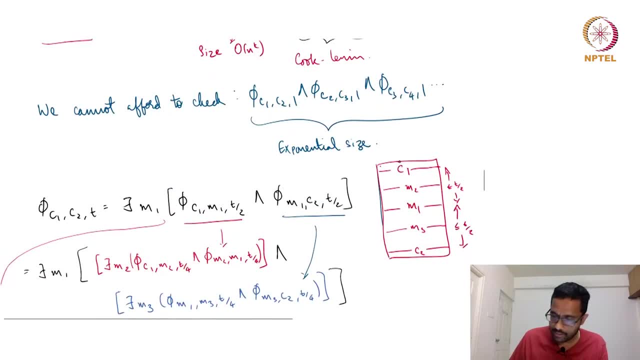 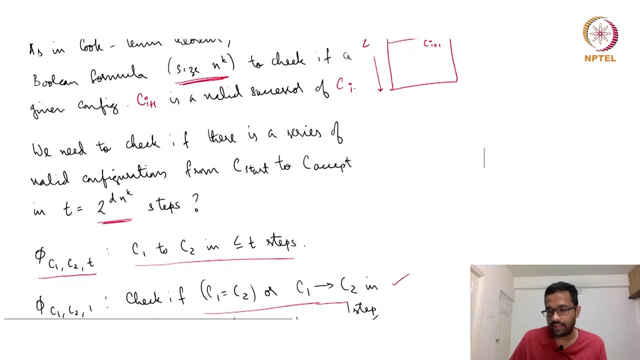 so the number of levels. So the number of levels is the number of levels, So the number height of the. so I am saying log h here, where h is the height of the computational table, which is 2 power d times n power k. So log h is the height of the computational 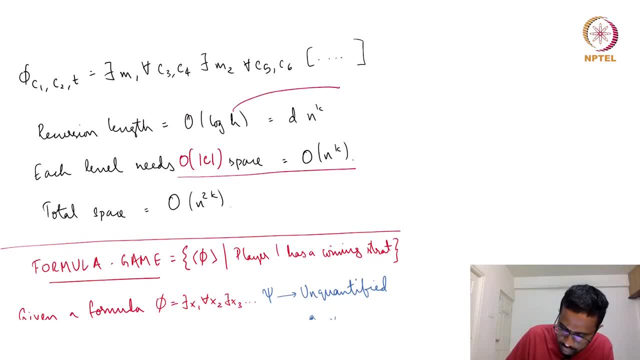 table. So where- maybe I will write that also- H is equal to height of computational table, which is equal to 2 power d times n power k. So when you take log of that, it is just d times n power k. So this is the number of. 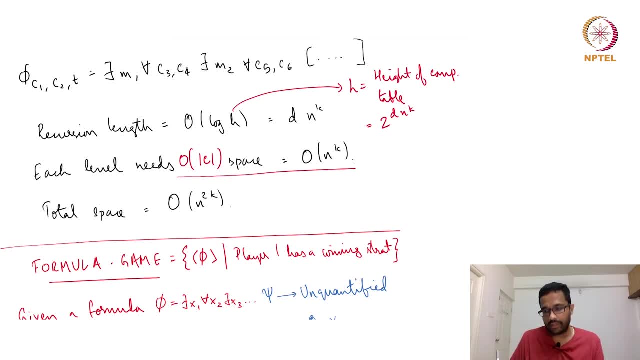 levels And at each level you require order n power k space. So the total space used is some constant times d power k- sorry, n power k multiplied by order n power k, which is order n power 2k with a constant. So it is order n power 2k. 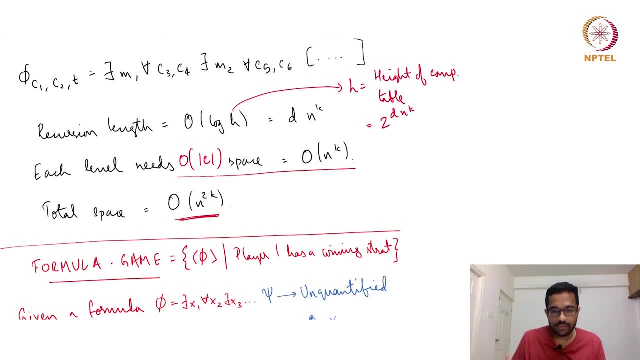 And this is the total space required to write down the formula. So this means that the this is the total space required to for the computation of the formula And even to write down the formula it is a similar amount of space. So this is the recursion length and 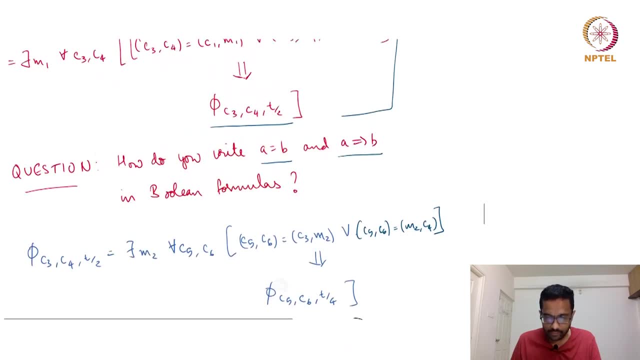 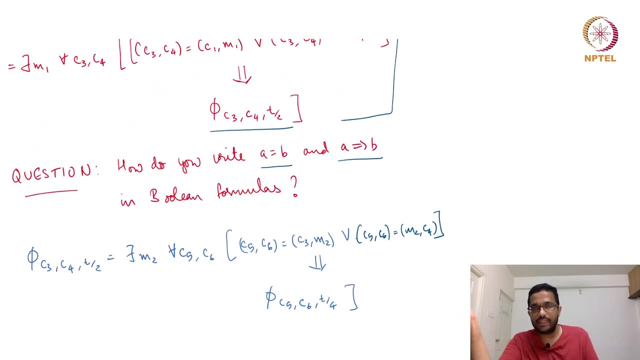 this is the number of space required. So hence, and the correctness is kind of evident, because, again we from our experience in the Cook-Levin theorem, this formula captures whether there is a, There is a sequence of configuration that need a string to be accepted, which happens. 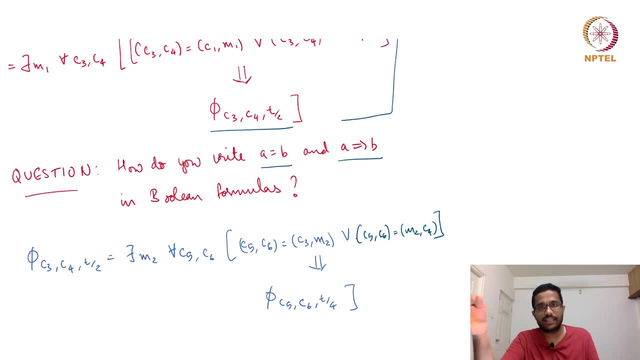 when the string is accepted by a machine, which happens when the string is in the language. So again, everything is if and only if. So the correctness of the reduction is evident. The time complexity is total, space is n power 2k and the time taken for the computations. 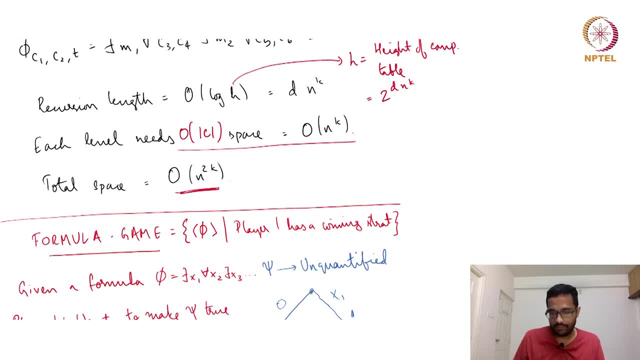 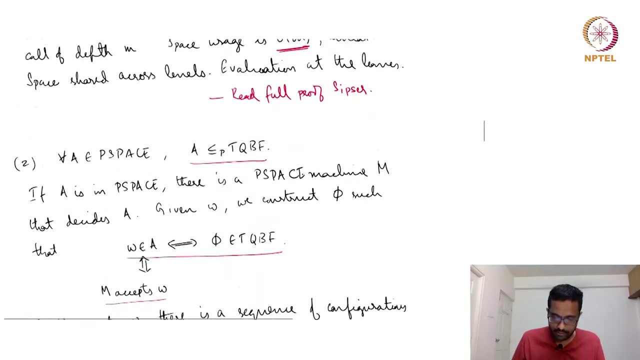 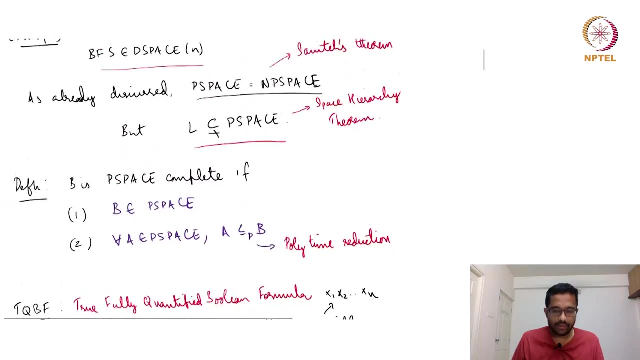 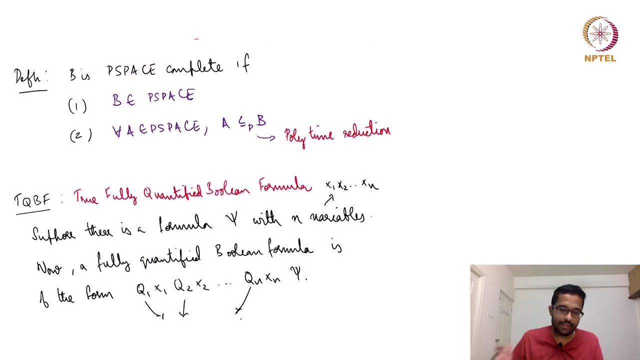 also this is a very structured thing. that is also is polynomial time. So So, just to summarize, just to summarize this, we defined what is P space, which is polynomial. it is a space analog of p. We defined P space completeness. again, it is. 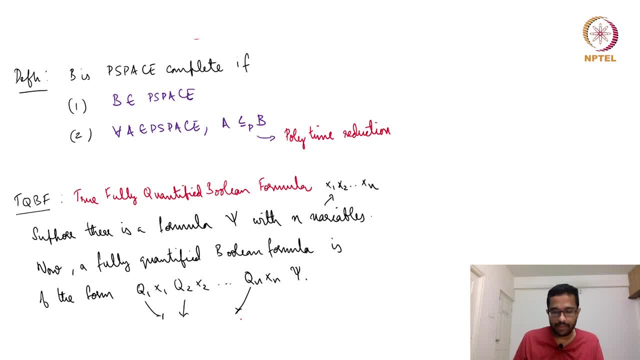 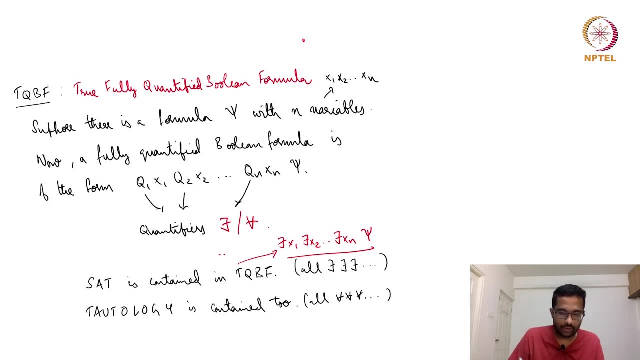 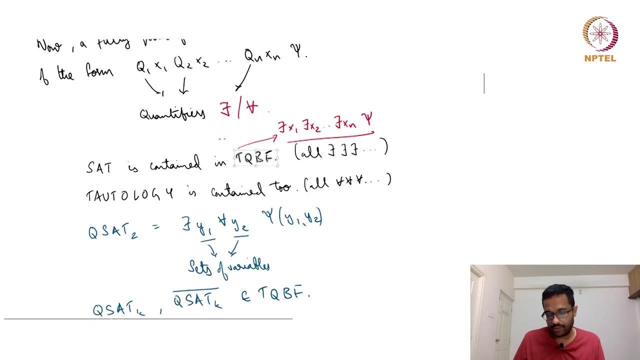 a space analog of kind of a space analog of N p completeness, and the first P space complete language that we saw was TQBF, which is short for True, Fully Quantified Boolean formula, where all the n variables are quantified. We saw that QSAT, 2, tautology, everything is. 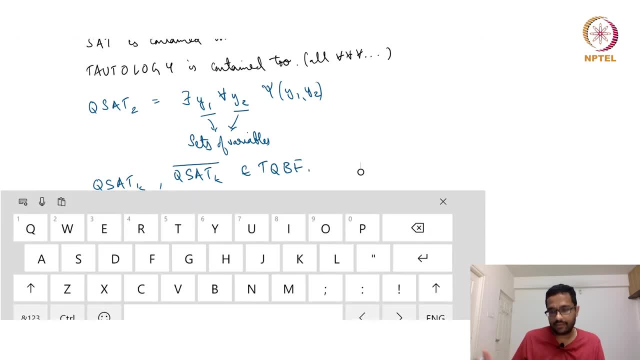 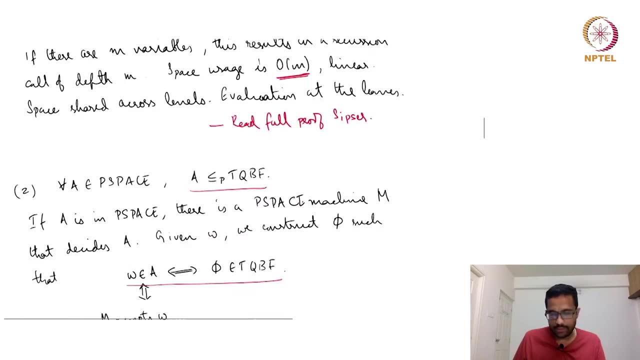 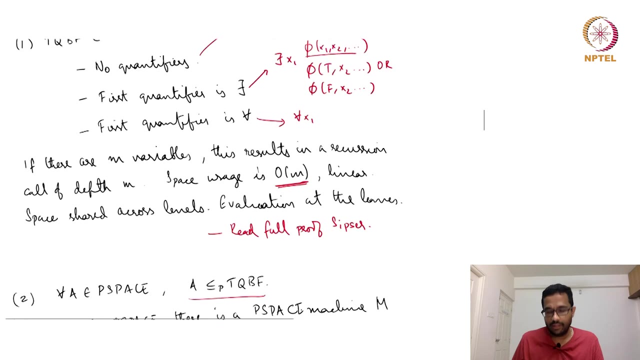 in TQBF. everything is a sub problem of TQBF And we saw why TQBF is PSPACE. complete the fact that TQBF in PSPACE is. it is rather straightforward And the proof that any PSPACE language can. 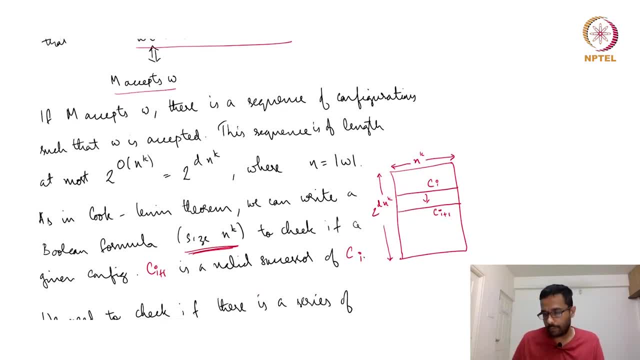 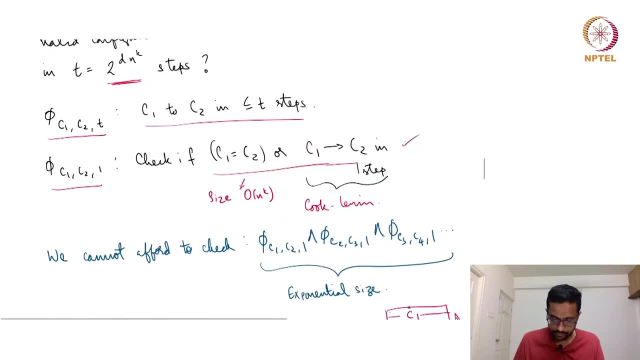 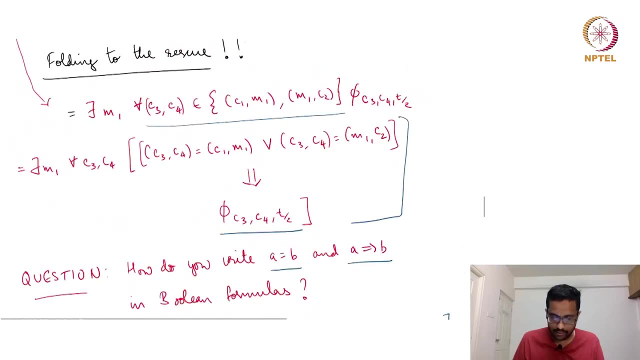 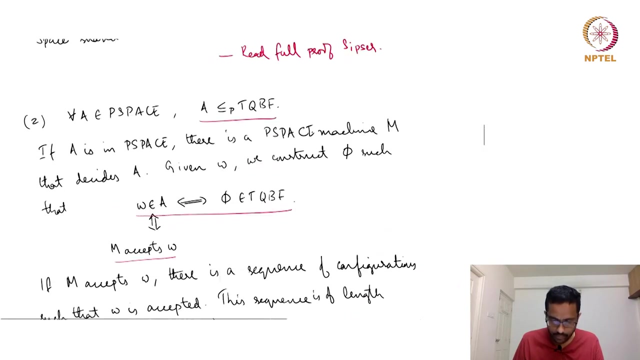 be reduced to TQBF requires us to go through computation table and some simplifications in the Boolean formula that encodes the configuration. And that is about it for this lecture. I will complete the rest of the PSPACE completeness in the next lecture. I just wanted to add one more thing. 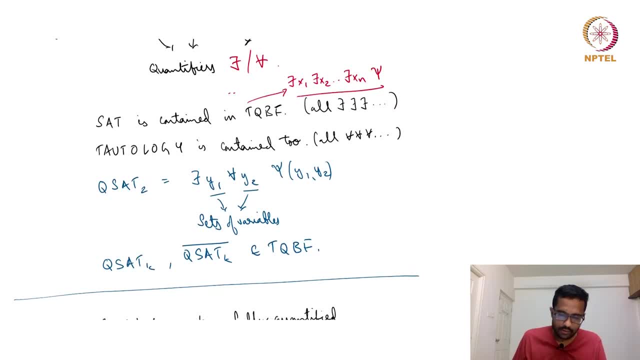 So notice that we are doing this under polynomial time reductions and we saw that SAT is contained in TQBF Tautology. is can be represented as a TQBF instance: QSAT 2, QSAT k, QSAT k complement. 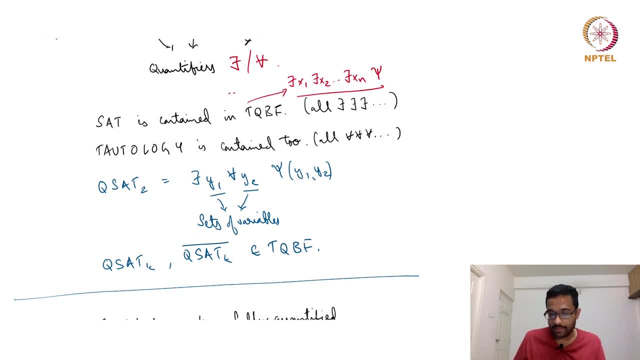 all of them are can be represented as a TQBF instance. This means that NP SAT is an NP complete language. all of NP can be is contained in PSPACE. All of co-NP tautology is a co-NP complete language. is contained in PSPACE. All of sigma. 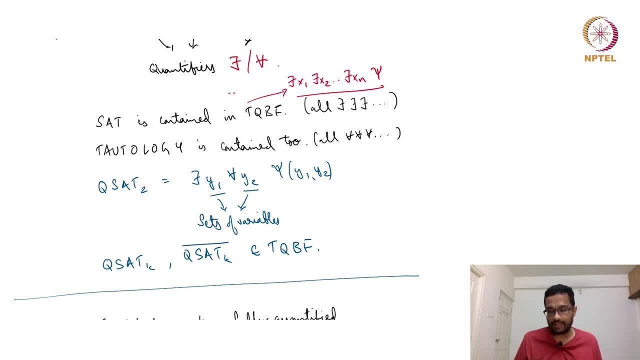 2 is contained in PSPACE. sigma k is contained in PSPACE. pi k is contained in PSPACE. So the entire polynomial hierarchy is contained in PSPACE. this is what it means. So think about this particular fact. So all of NP co-NP, sigma 2, sigma k, sigma k are contained in PSPACE. So all of NP co-NP. 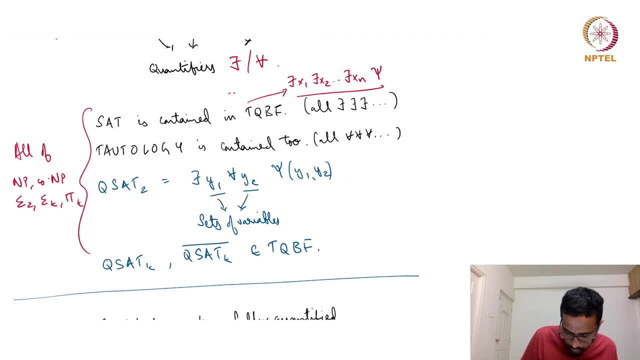 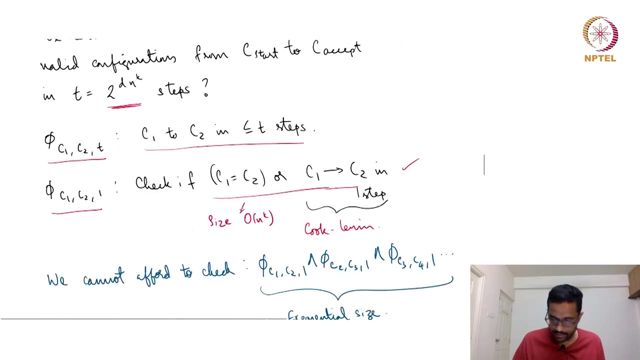 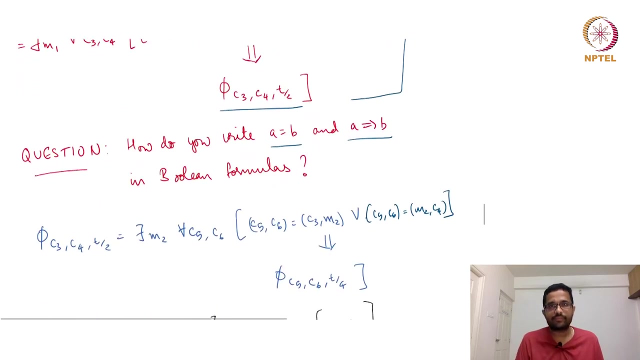 sigma 2, sigma k, pi, k, all are contained in PSPACE And with that thought I think I will close this lecture. In the next lecture we will see a couple of more instances of PSPACE, complete languages. Thank you.